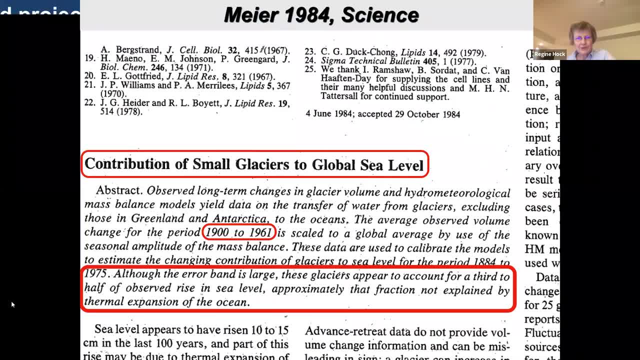 and the projections of global glacier mass changes. Mark Meyer was the first to recognize that these glaciers outside the ice sheets may play a significant role in global sea level rise, And he wrote here this paper in 1984, concluding that between 1900 and 1961, the glaciers contributed. 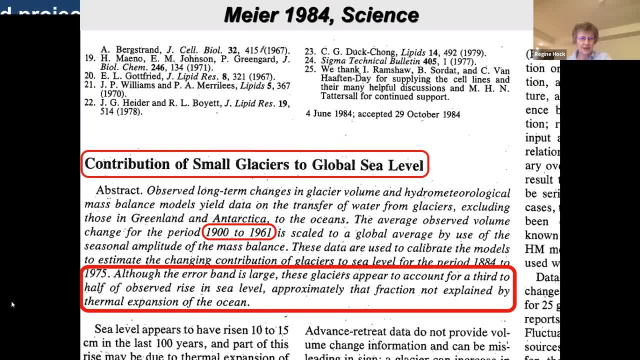 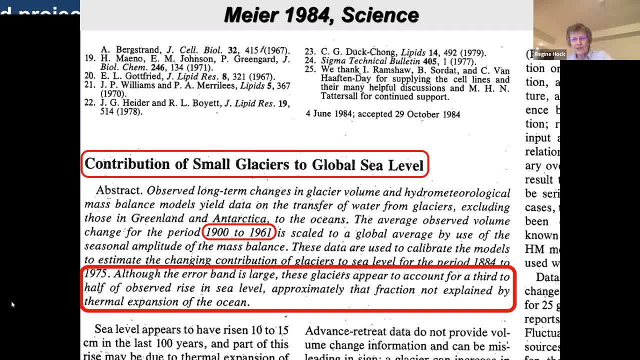 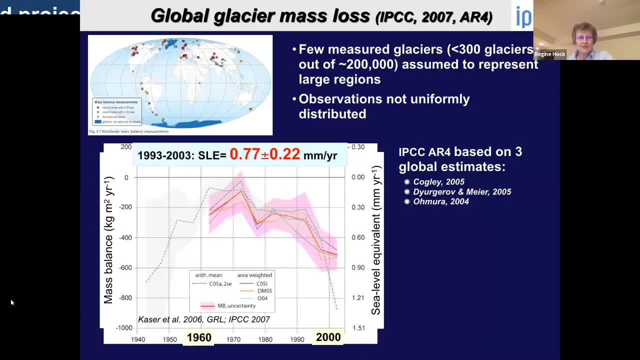 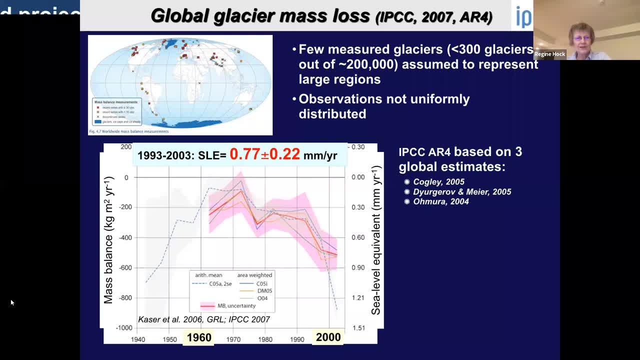 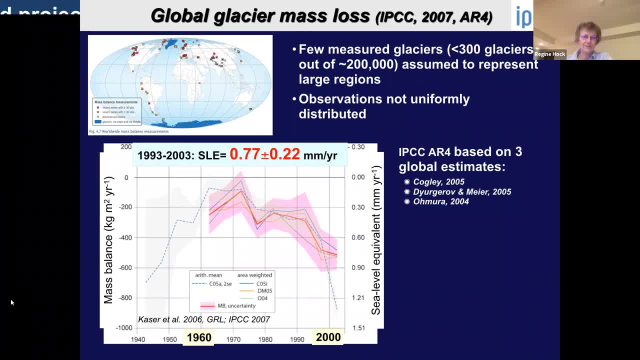 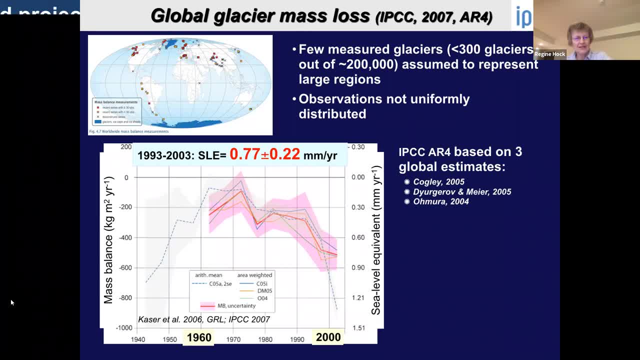 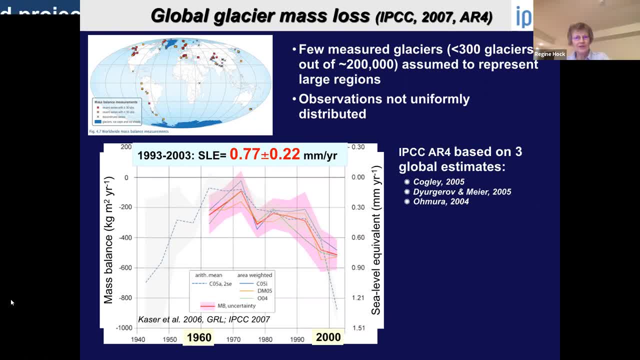 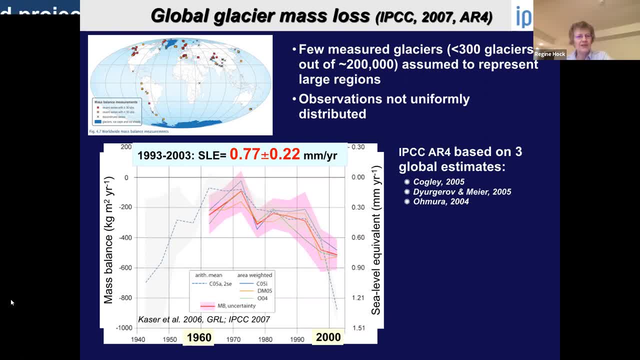 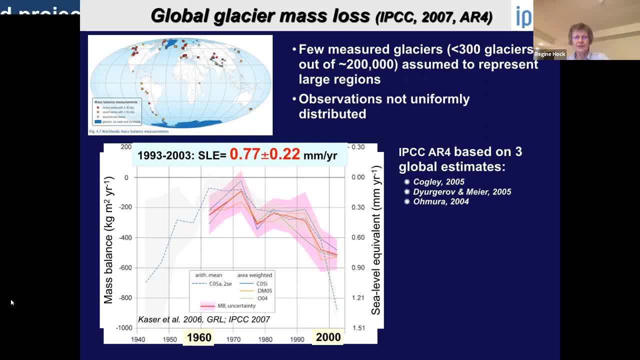 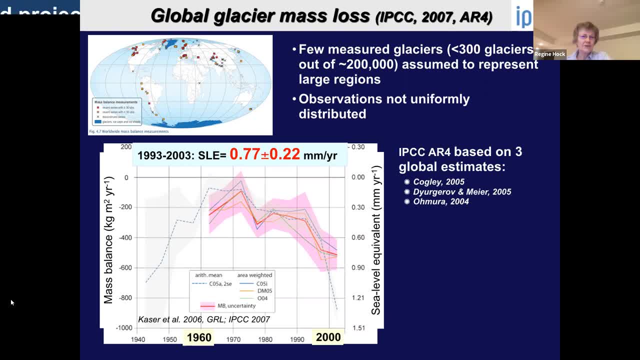 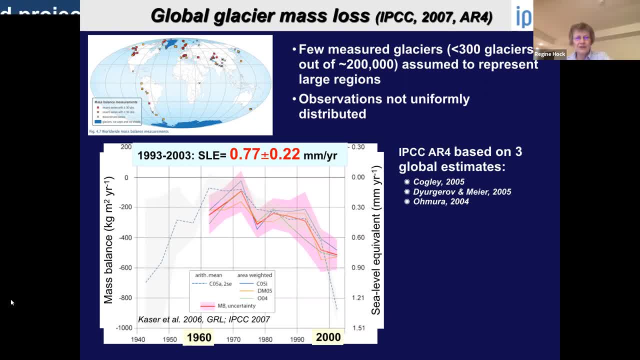 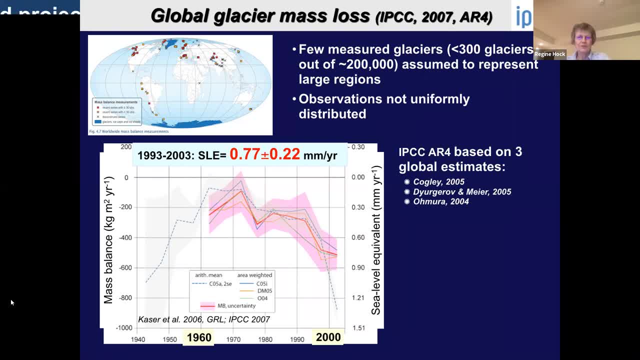 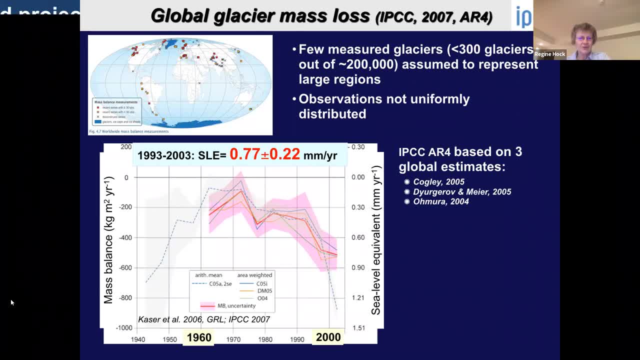 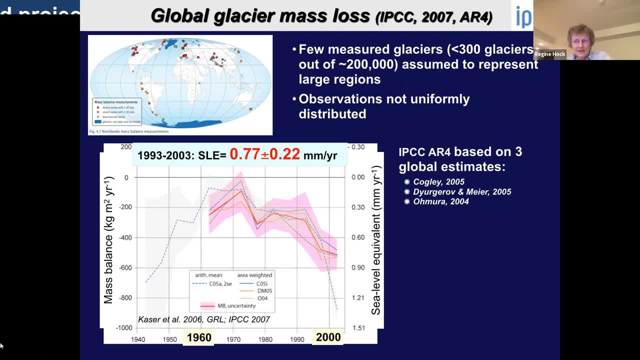 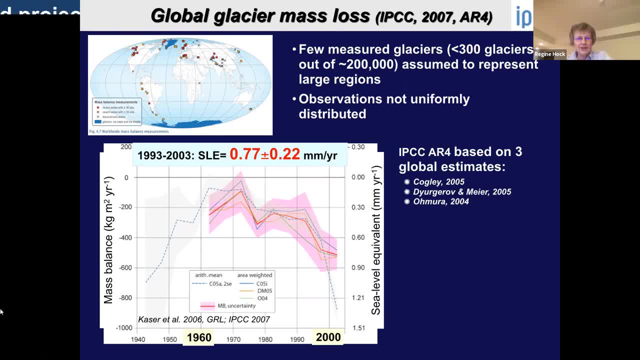 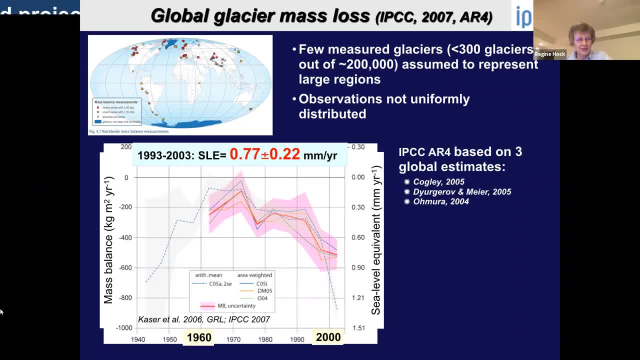 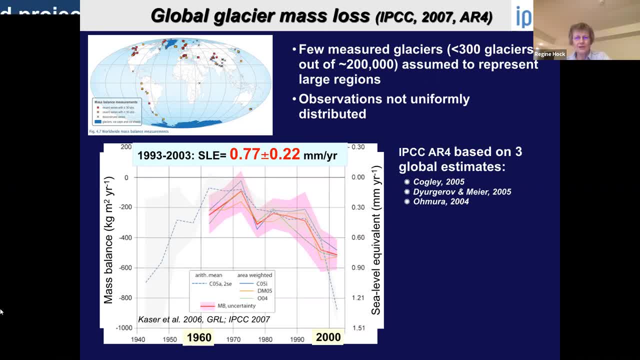 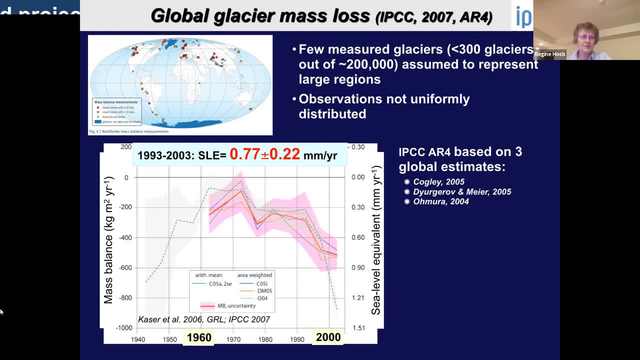 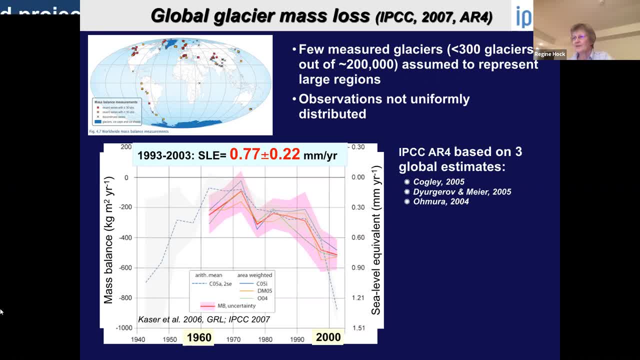 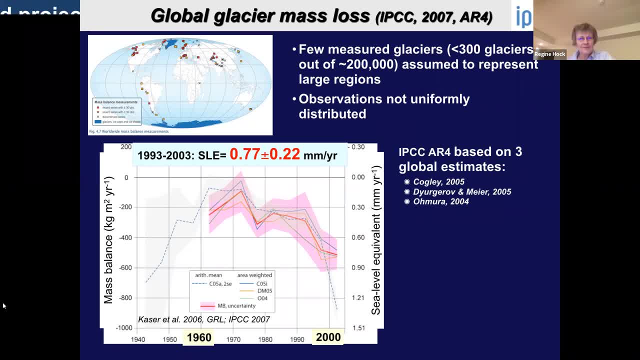 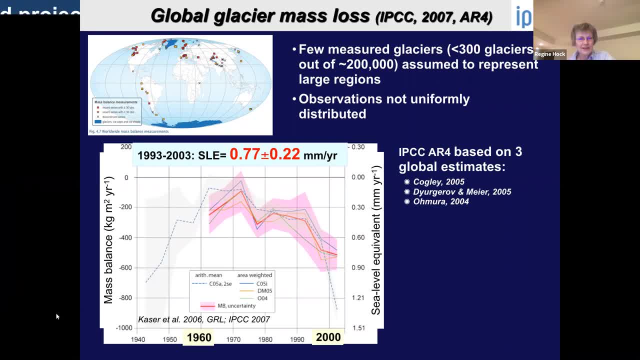 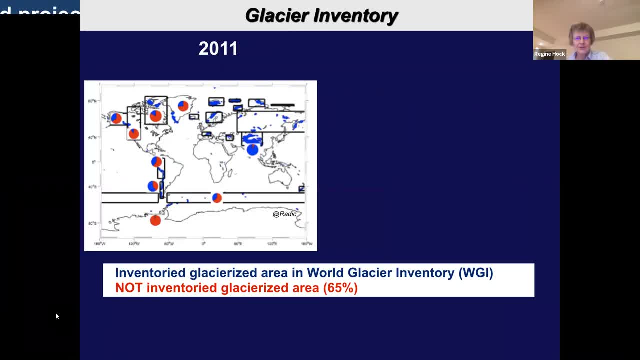 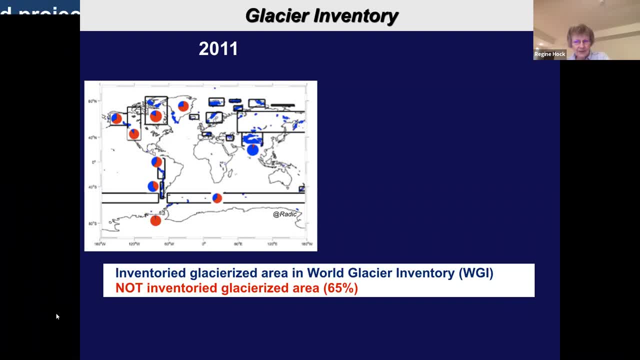 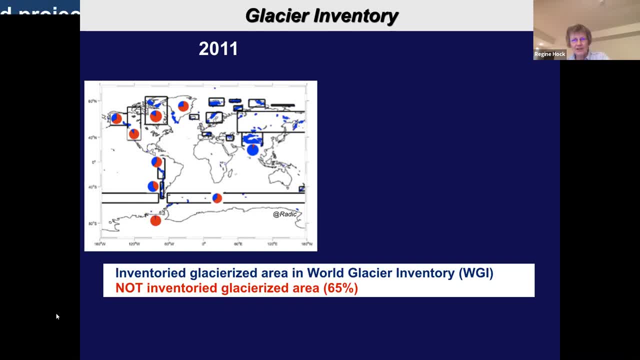 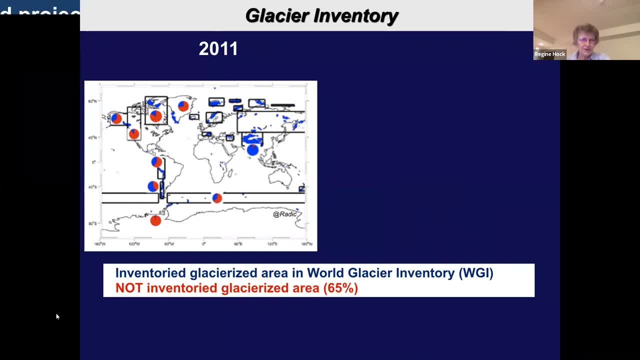 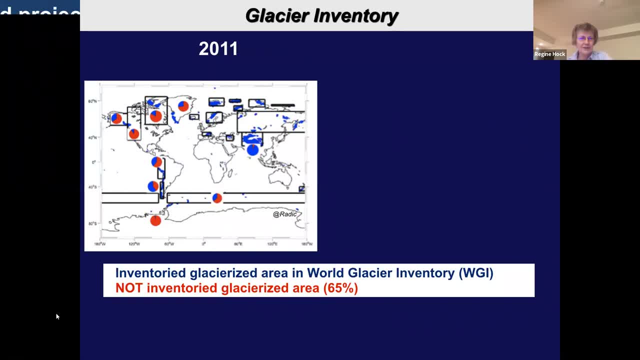 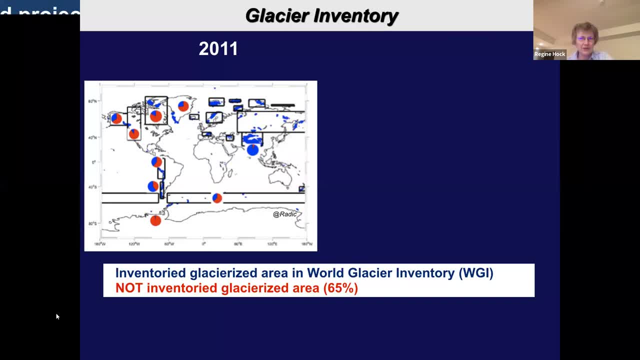 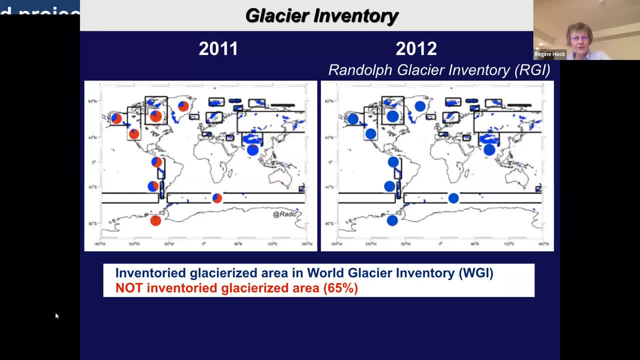 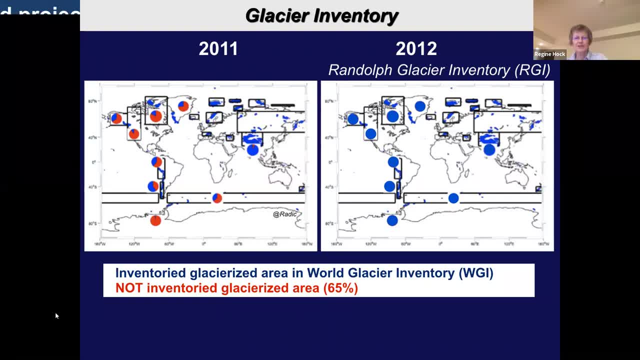 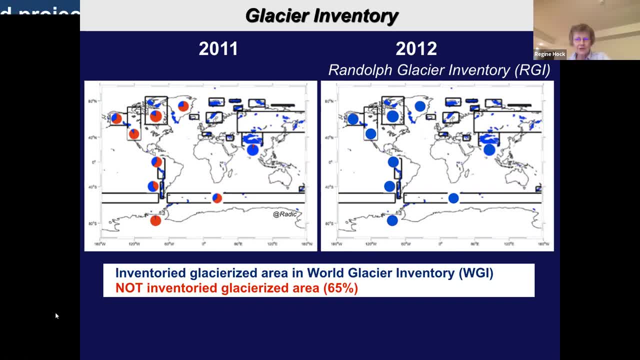 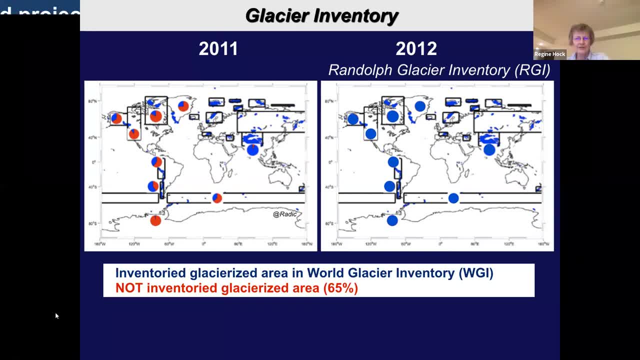 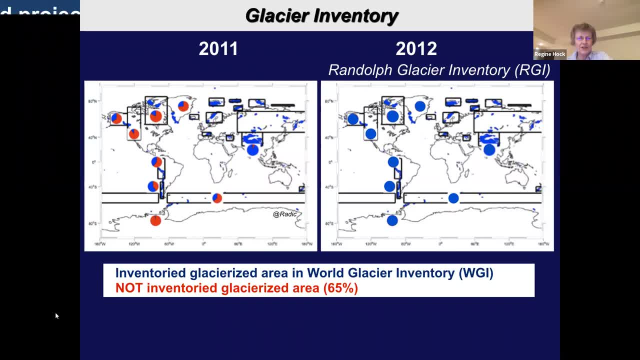 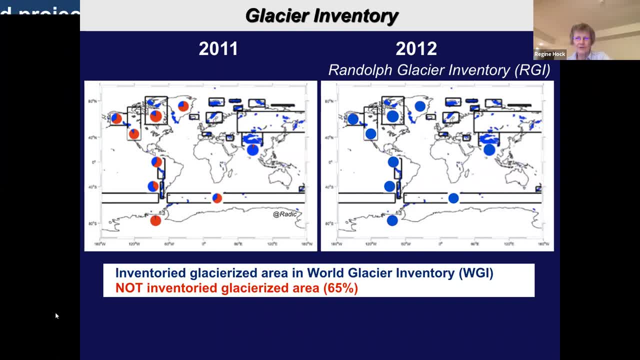 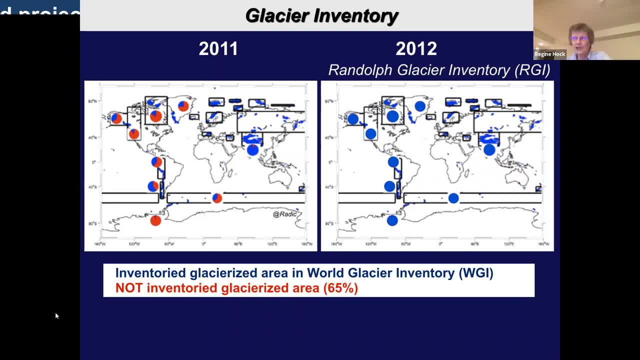 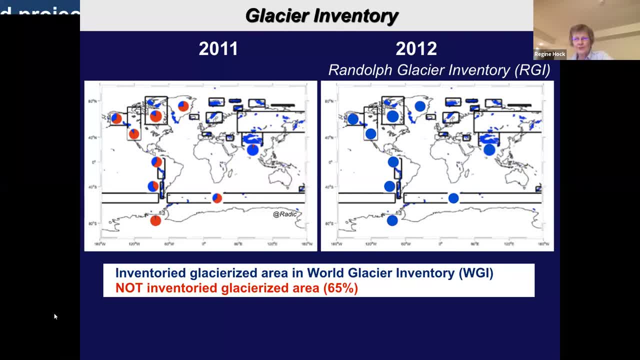 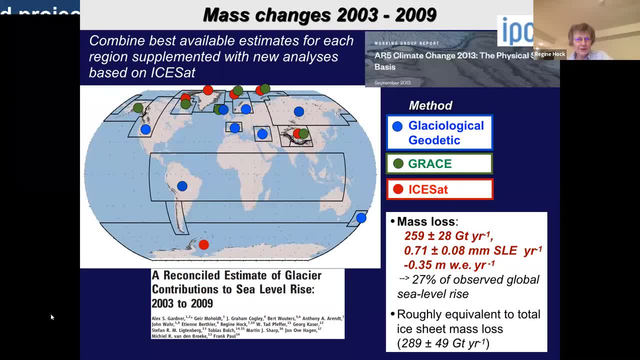 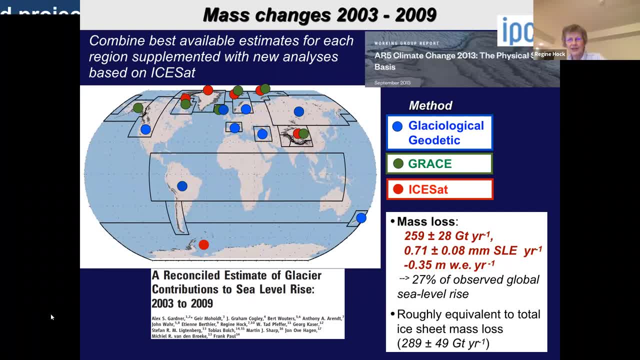 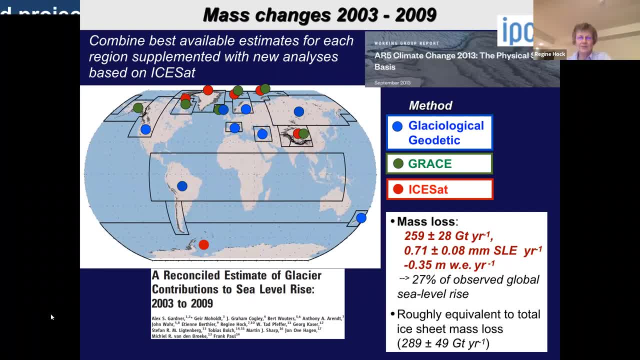 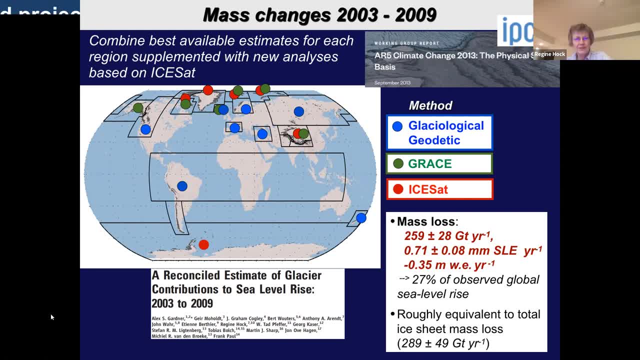 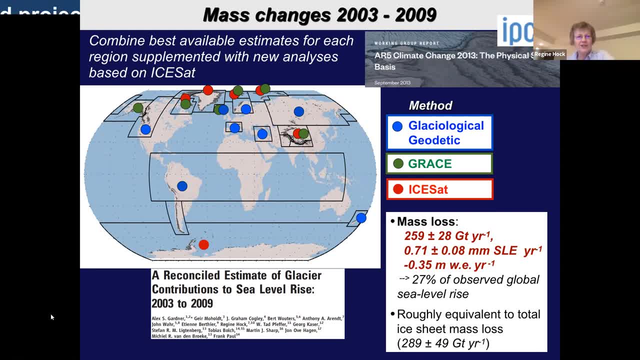 These estimates were, of course, global sea level rise. I think you answered that right. Here are the fields around the map. The region showed other data of global surface changes. The other distribution of the glaziers to sea level rise, about 0.71 millimeters during this period here. Since AR5, only a very few more global scale mass change estimates have been published Here: the one by Tsempt et al, based on glaziological geodetic measurements. Now a lot more data went into the extrapolation, but still in many regions 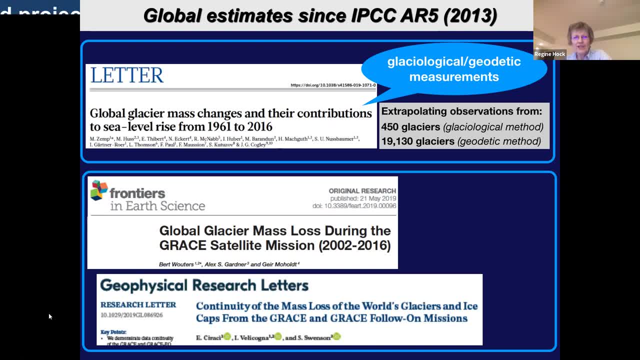 especially the ones where there's a lot of ice in the polar regions, were not well covered. Often only like less than 5% of the area was covered in this estimate. And then they also were like two new global scale GRACE estimates. 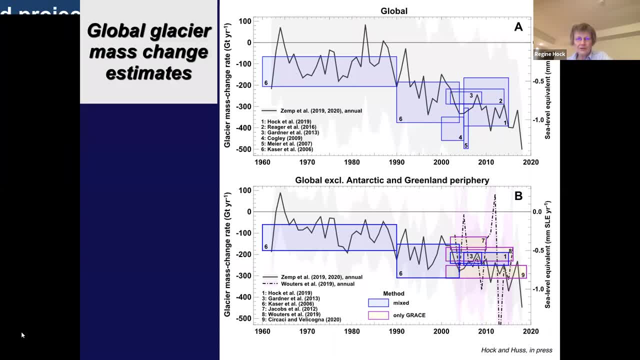 What you see here is a compilation of all available global mass change estimates. So the upper panel shows all glaziers, including those in the Antarctic and Greenland periphery Below. it's excluding those glaziers and we show them separately because there's far more estimates. 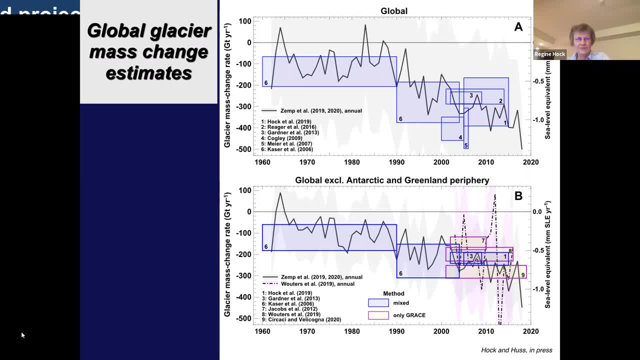 if you exclude the Antarctic and Greenland periphery. The black lines show the annual mass changes by Tsempt et al, based on extrapolating glaziological and geodetic observations. The gray is the uncertainty. The boxes are multi-year means over different time periods, and 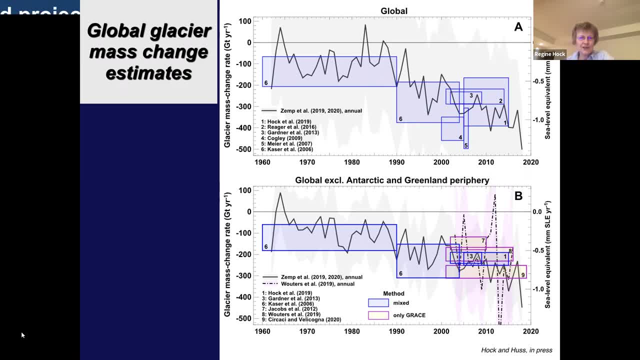 in the vertical is plus minus the reported uncertainties, And pink marks the estimates by GRACE. What you see here is more negative mass balances in the last part of this period. Also, you see large differences between different estimates, some of them not even overlapping within uncertainties, although they cover more or less similar periods. 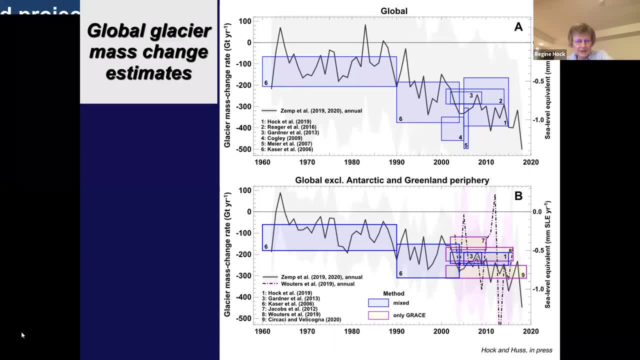 Also large discrepancies between the GRACE-derived year-to-year variability, shown here in pink, and the annual balances derived from the glaziological observations, And it became clear that looking at these differences here that the community needs to get together and try to understand these differences and tackle the mass change. 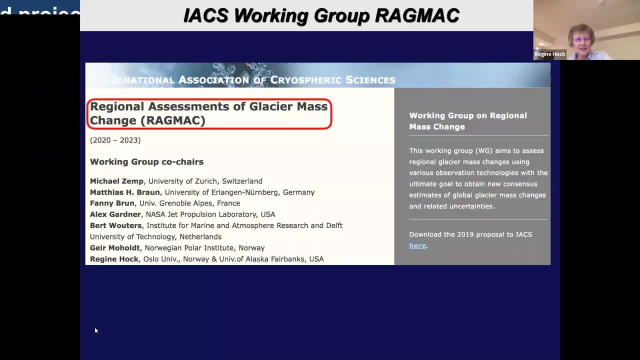 assessments in a more coordinated way, And this has led to the recently established working group of RACMAC by the International Association of Cryospheric Sciences. IACS and RACMAC stands for Regional Assessment of Glacial Mass Change, And the goal is to work towards improved mass change estimates and 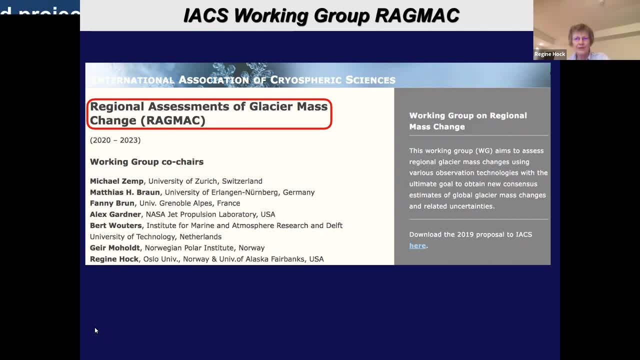 come up with best practices for these different methods, to derive global estimates from the glaciological, geodetic and gravimetric methods and really try to understand why we have all these differences and how we can reconcile them between the methods. So much about the past. Now I want to move to the future. 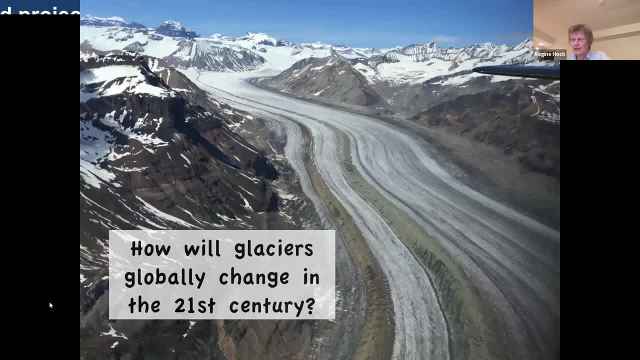 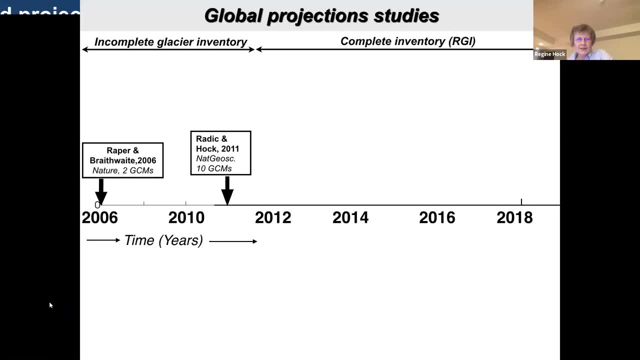 How will glaciers globally change in the 21st century? And also here I want to give a little bit of a historical perspective Over a period of more than a decade. only two global scale projection studies can be found in the literature, And as for the past assessments, a huge problem was that the inventory was incomplete. 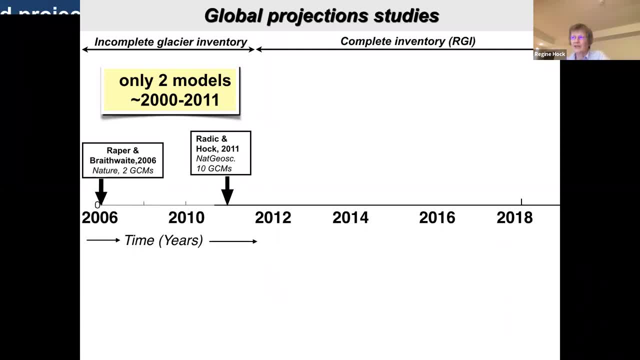 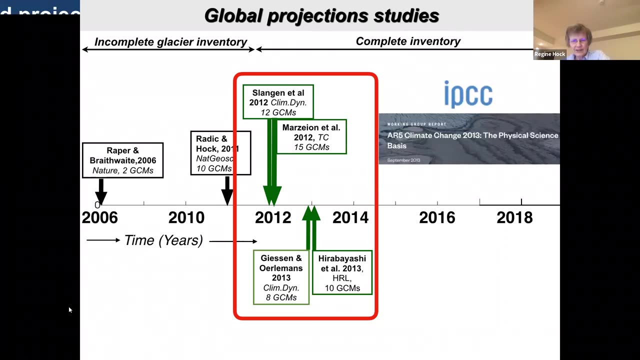 And that's probably also a reason why there's not too many other studies, because it was just very difficult to make projections if you don't have a complete inventory. This changed then with the new complete RGI inventory and with IPCC coming up, a few new models were developed. 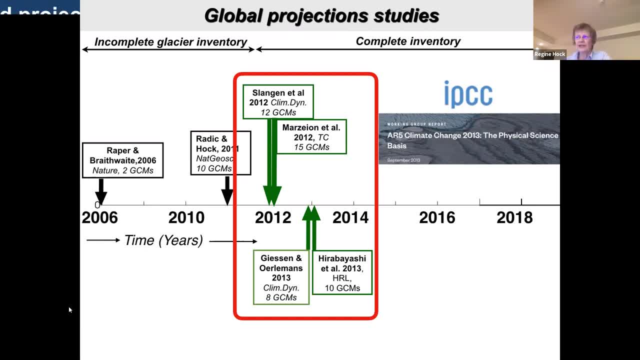 But still, I want to emphasize, within almost 20 years, there's just six published studies that project glaciers on a global scale. So that's a very, very different than in the ice sheet community, where there's really a lot of models projecting the future. 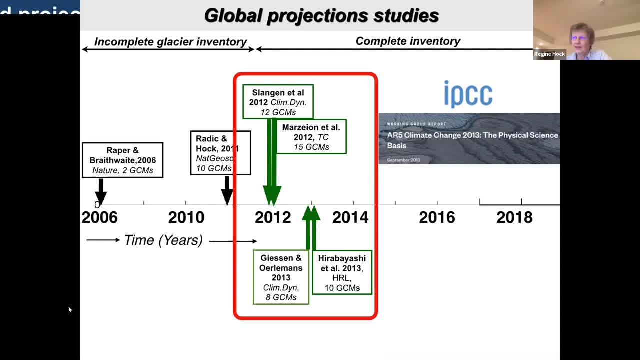 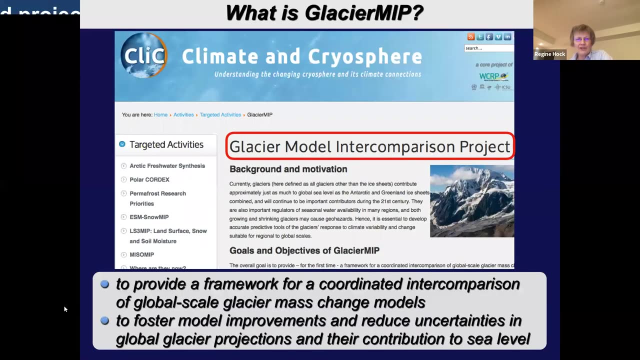 None of these efforts here, of these studies, was coordinated with any other groups. It was just sort of single studies published by different groups in the world. So we saw also here a need for more coordinated effort and that's what Glacier MIP is about and that was started five years ago. 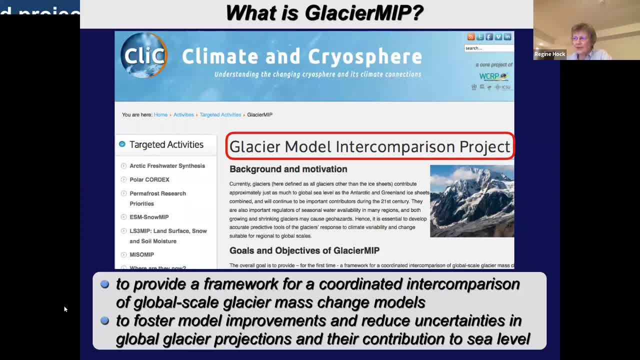 Glacier MIP is the glacier model into comparison project. Glacier MIP is the glacier model into comparison project. Glacier MIP is the glacier model into comparison project. It's a targeted activity by CLIC, the Climate and Cryosphere Project, and the goal is here to provide a framework for coordinated intercomparison of global scale glacier mass models. 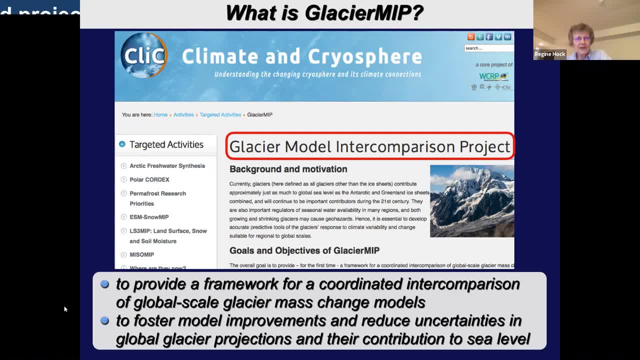 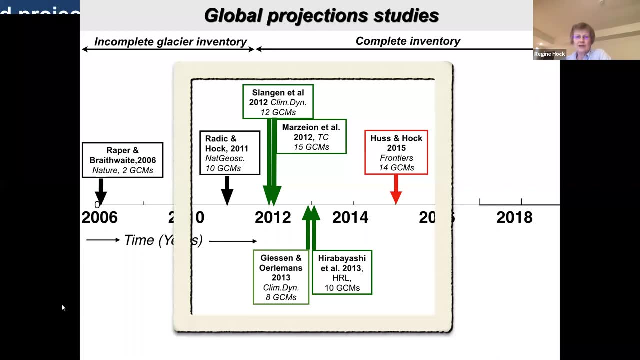 mass change models and also to promote model improvement and try to, in collaboration here, to reduce uncertainties in these global scale projections. And as a first step, the first step was to take the studies that were in the literature by that point in time- by 2016,- and compare the projections in a coordinated way. 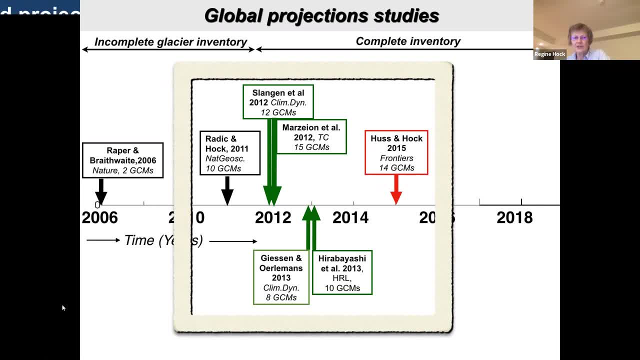 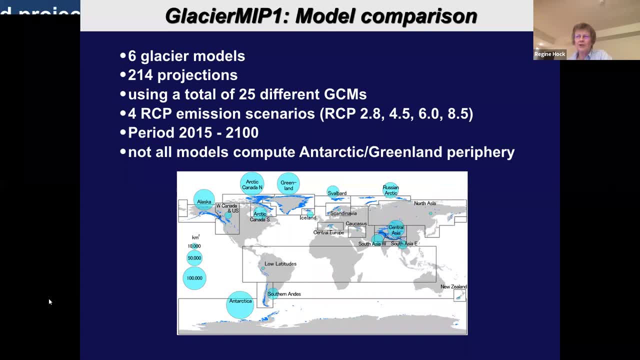 So these were the six models. it was an open call, so these were the six glacier models that submitted their data to Glacier MIP phase one. We had a total of six glacier models- 214 projections. We had a total of six glacier models, 214 projections. 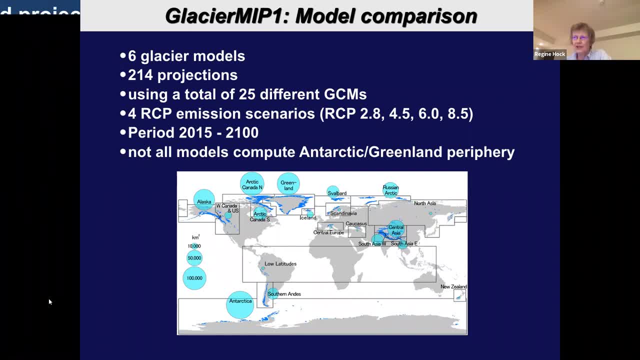 We had a total of six glacier models, 214 projections, Each of them using two to 14 different GCMs. in total, 25 different GCMs were used for emission scenarios and we looked at the period 2015 to 2100.. 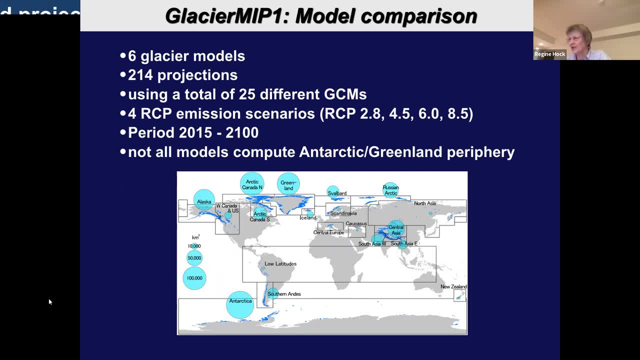 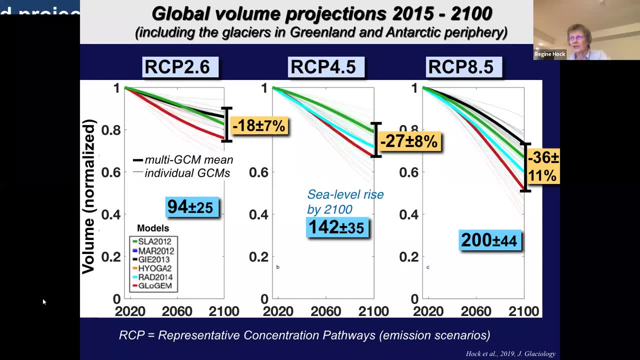 And all models computed all the regions here the RGI regions, but not all models computed the Antarctic and Greenland periphery. So here you see the results of the global volume projections. The silos were noisy but not all of them were very dramatic. 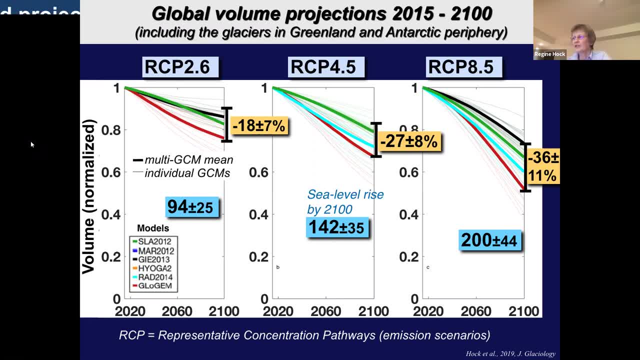 The videos show volume and regression from relative to 2015.. So one here means a hundred percent mass in 2015, and you see how much mass is remaining by the end of the century. The thick lines show the mayoría. GCM means arv, the different legit models, and the thin lines the individual GCMs. So results show – I mean substantial reduction in volume as expected, ranging here fromWe did be interested in at least 18 to 36% households. specifically inGoodlands We did be interested in at least 18 to 36%乳g, some sum of GCC, MIP, EVs and I think in general we have some ground tests there and we're glad to add that it got a lot of applications. 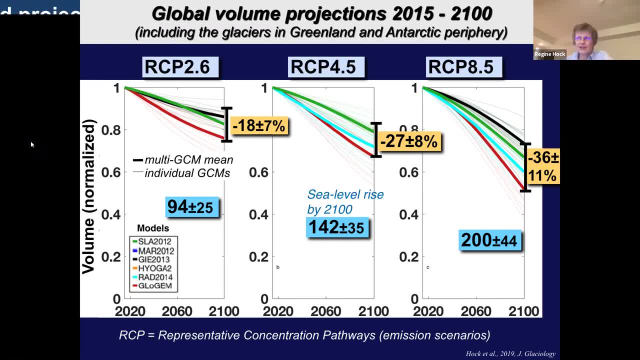 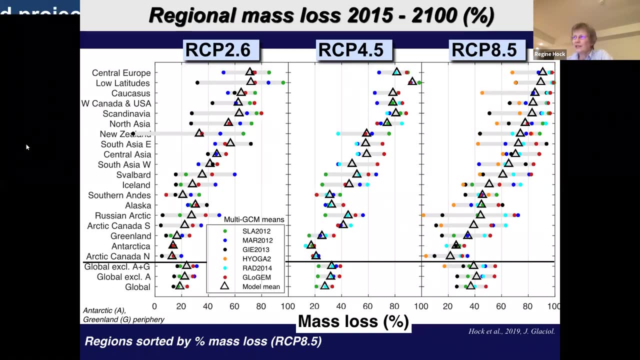 the mean for the different emission scenarios And the corresponding sea level equivalent is about 94 millimeters to 200 millimeters. This is on the global scale. The next slide shows here the regionally differentiated mass losses by 2100, the mass loss in percent relative to 2015.. 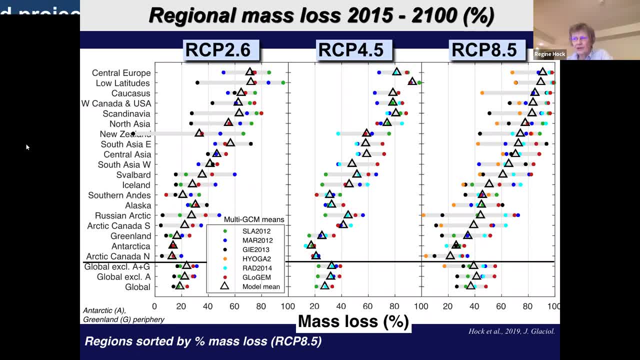 You see here the 19 RGI regions, and the lower three rows show the global scale, with or without the Greenland and Antarctica. The regions are sorted by percent mass loss And what you can see is there's huge differences between the regions. the regions that have little ice. 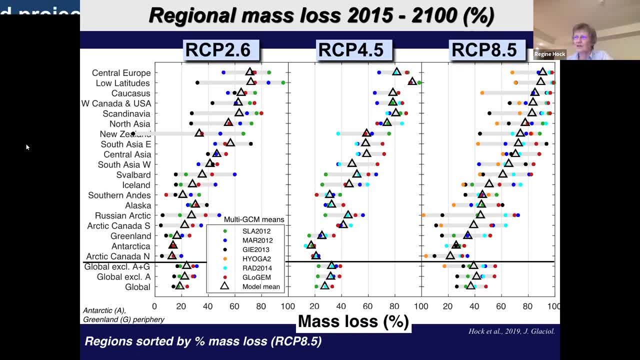 like Central Europe or Caucasus or Western Canada, lower latitudes. They have large mass losses, up to like 80, 90% by the end of the century, whereas the regions where there's a lot of ice it ranges between 20, 25, 30% mass loss. 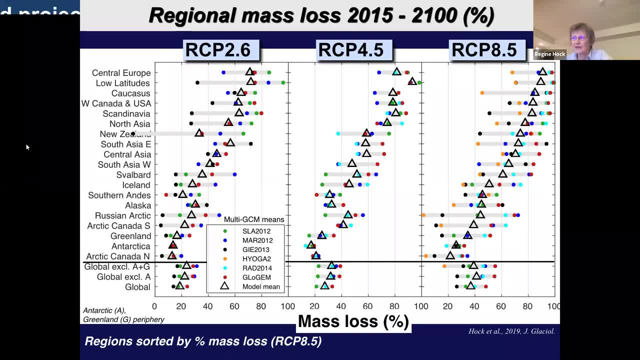 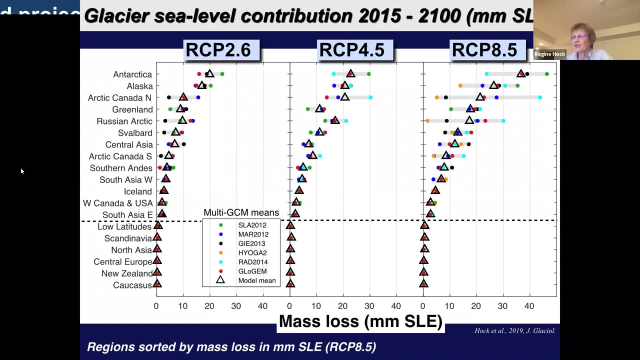 So each of the dots here is a multi GCM mean of one glacier model. This is the relative mass losses, but of course for sea level what matters is the sea level contribution, And here also now ordered by mass loss in millimeter, sea level equivalent. 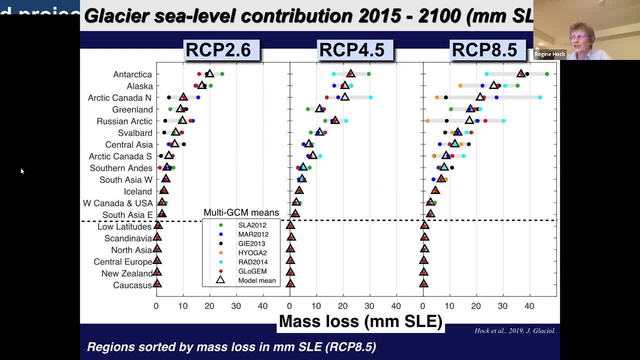 And here you see that it is really only a few regions that contribute most of the sea level rise, The regions with a lot little ice. down. here they contribute very little, whereas like Alaska, the Antarctic, Greenland periphery Arctic, Canada, Russian Arctic. 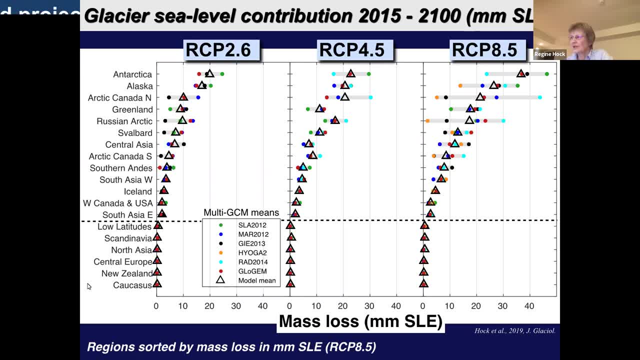 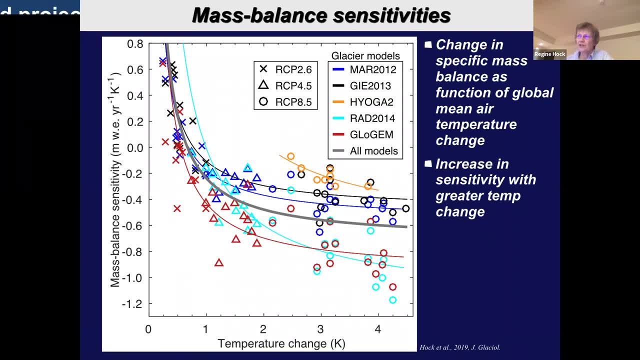 are the main contributors to sea level rise. We also looked at the mass balance sensitivities. So the mass balance sensitivity defined as you know, the mass balance sensitivity defined as you know, the mass balance sensitivity defined as you know, is how much will the mass balance change? 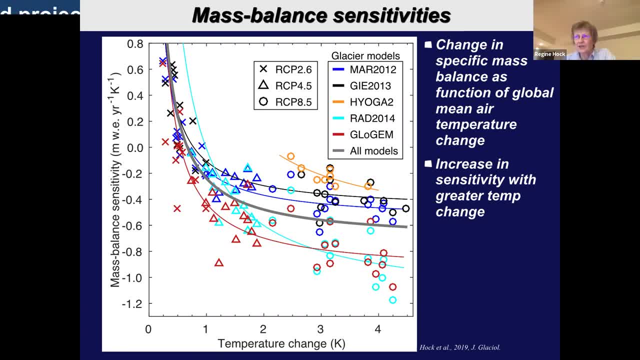 if temperature increases. So it's really the change in specific mass balance per degree temperature increase And to see this here as a function of global mean air temperature change, that was extracted from each of these ones And what we see here is an increase in sensitivity. 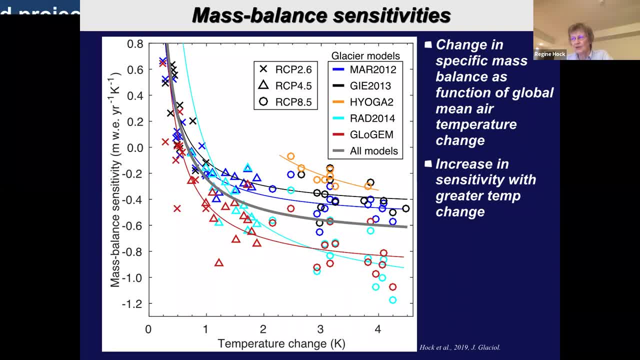 with greater temperature change. So the sensitivity is not constant. It changes as a function of the temperature change. You also see differences here between the models, that some models have a higher sensitivity than others, And that's of course important. So you want to really understand also these differences. 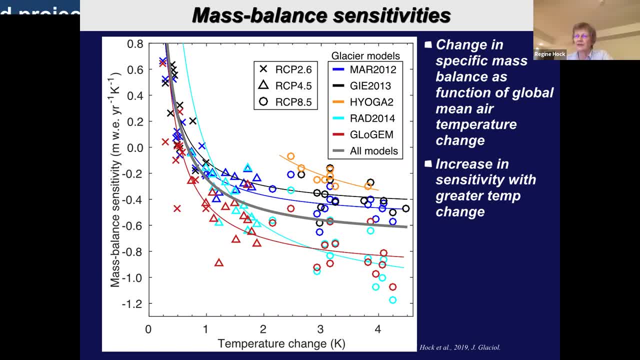 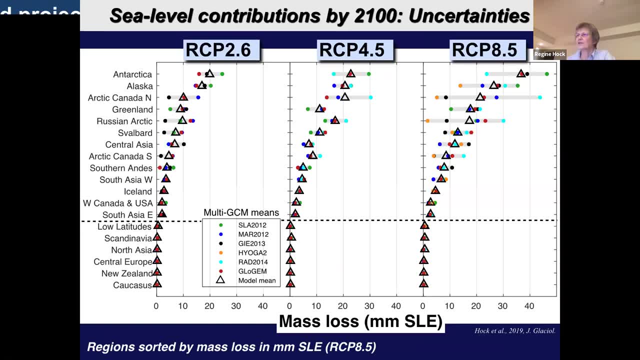 in the projections that we see here that they- yeah, the models have different sensitivities. Going back to this slide here to the sea level contributions by the end of the century, it is the regions where it matters most here up here. 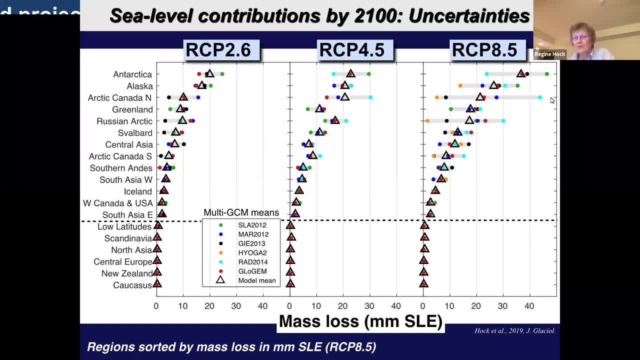 and Arctic, Alaska and so on. That's the regions where we have the highest uncertainties, the largest differences between the different Glacier models, And that's, of course, a problem. These experiments were not standardized, So part of the reason is, of course, that each of these Glacier models 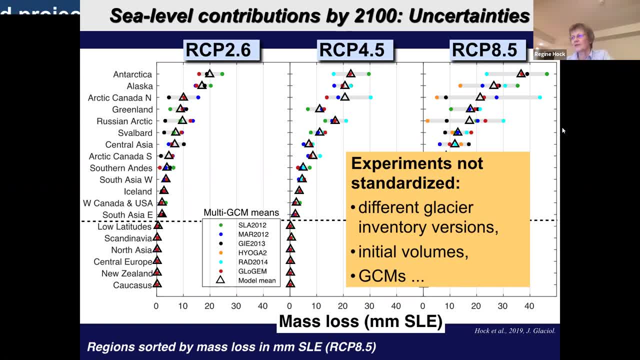 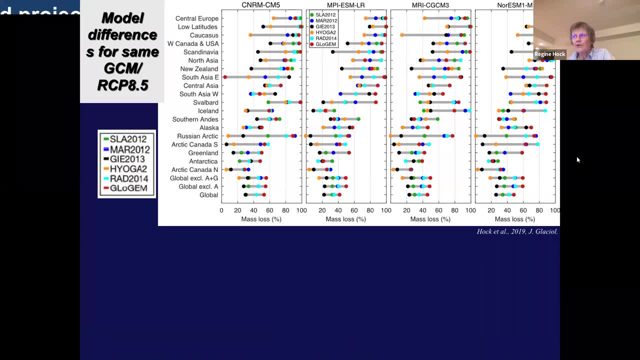 use different Glacier inventory versions. They use different initial volumes, different GCMs, So they are not directly comparable. But for four GCMs you can directly compare them. So to eliminate those effects of different ensembles we looked here at simulations that use exactly. 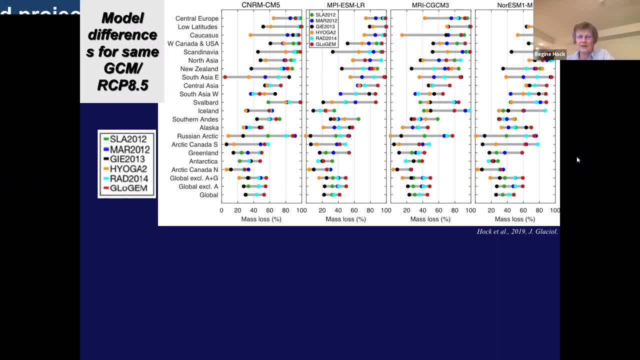 the same GCM and the same emission scenario And there were only four GCMs that were used by all Glacier models And when we look at those we see substantial differences in the percent mass loss by 2100 between the Glacier models. 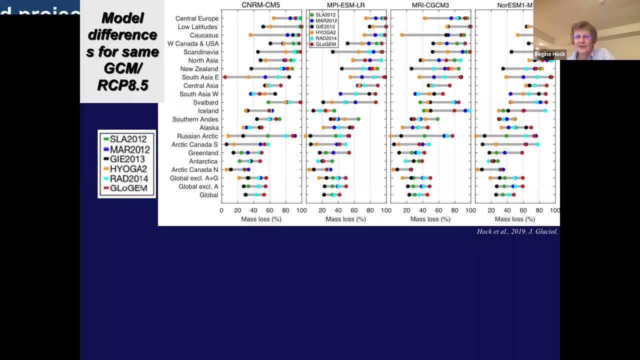 Ideally these dots should be all on top of each other And interestingly these differences are not necessarily systematic. For instance, one Glacier model model may project the lowest mass loss in one region but a higher mass loss than the other models in another region. 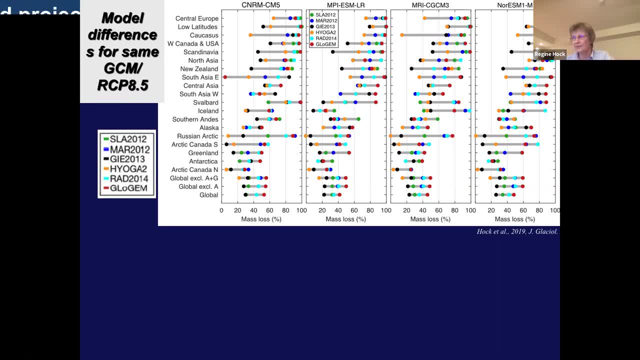 So they do have not only different sensitivities when you compare the Glacier models, but it differs actually. it varies from region to region. I wanna just highlight here three regions where it's I mean dramatic differences, like the Russian Arctic. one Glacier model predicts no change. 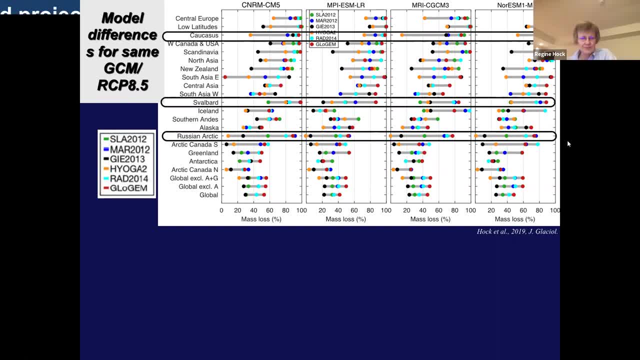 and another one about an 80% mass loss. So this is, of course, a problem, and we need to understand why these models have such different sensitivity and behave in such a different way, And possible causes for these differences are the different region boundaries that they use. 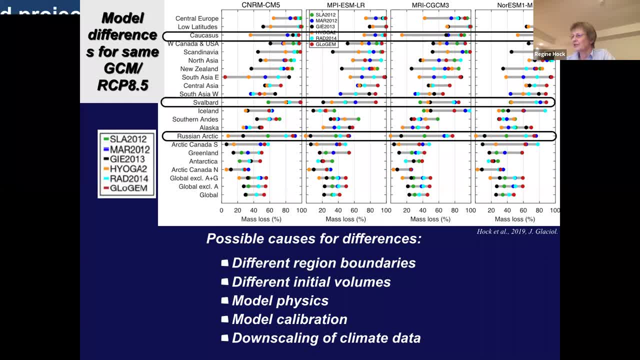 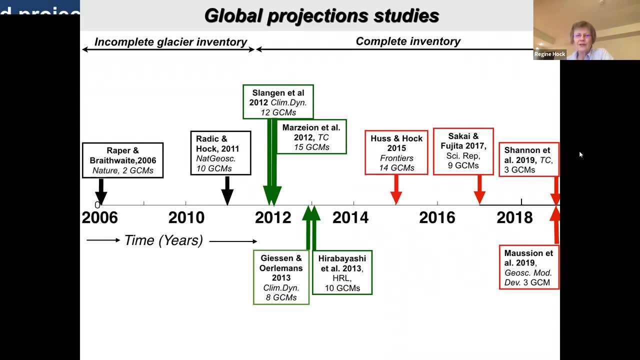 the different initial volumes, but also differences in the model physics, how they were calibrated and how the climate data was downscaled. So since AR5, a few more models were published. Here are the ones in red. And so for the next phase of Glacier MIP, 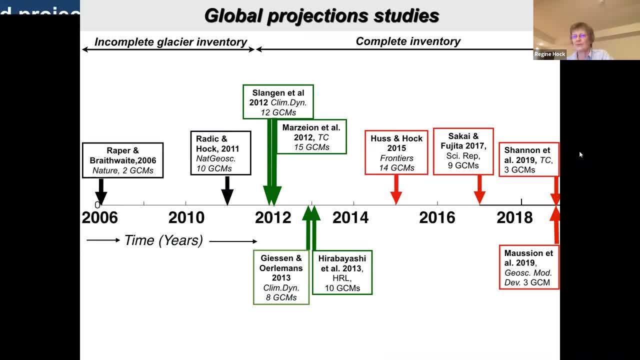 after this comparison of existing previously published projections- the ones here in green- and we wanted to provide the community-based consensus projections for the upcoming IPCC AR6 report. So we saw a need for more standardized approach and standardized projections for the next phase of Glacier MIP. 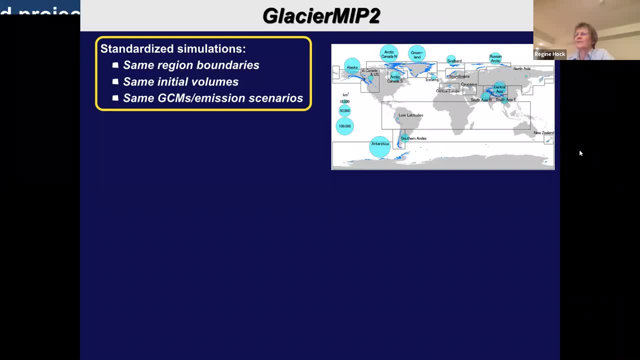 So we had an open call for participation. We prescribed the boundary conditions here: same region boundaries, same initial volumes, same GCMs and emission scenarios- and all modeling groups had to adhere to those. There was a total of seven, 11 Glacier models. 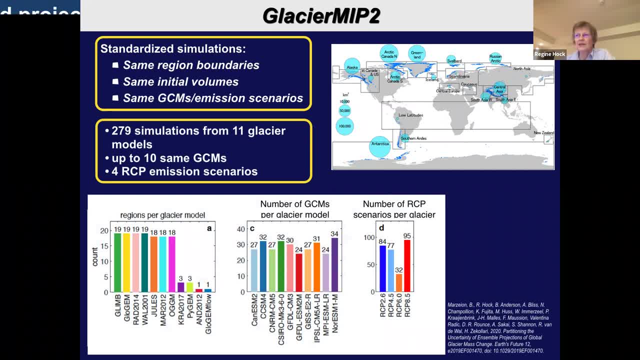 So the community has grown and we had about 280 simulations. We prescribed up to 10 GCMs. Not all of them used all of them, but yeah, those were the 10 that were we all used and four RCP emission scenarios. 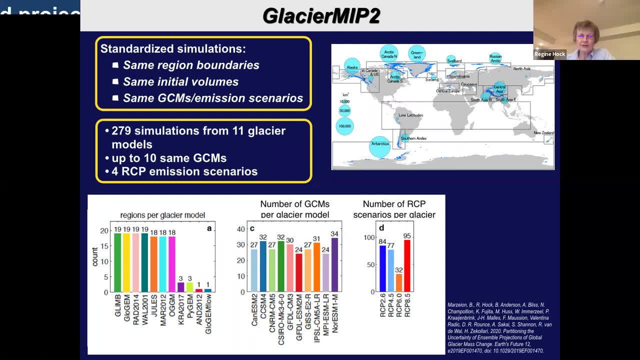 of the 11 models, four took part in the previous comparison and there were seven new models And the ensemble was richer this time in terms of model physics. So some of the models included our energy approach, air balance approach or flow model. 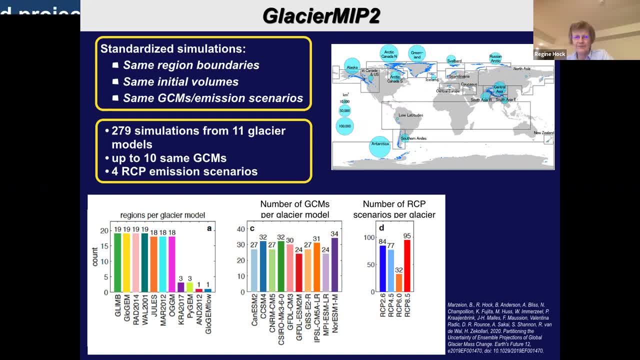 And we also had one earth system model participating here. So for the first time it was a much more coherent ensemble of projections, even though, as you can see, it's not the number of GCMs per Glacier model for the ensemble, but it's not exactly the same for all. 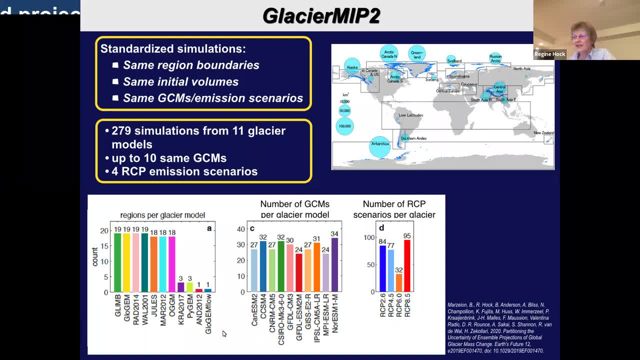 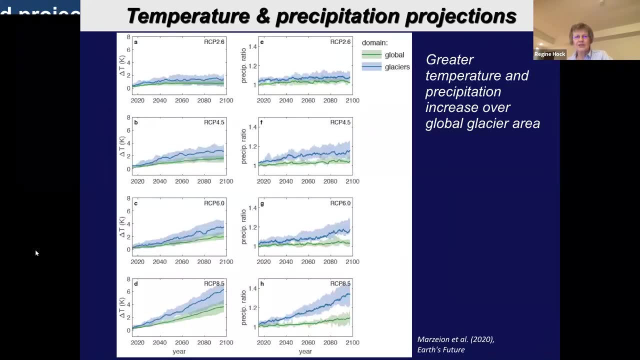 also not all used all the RCPs And some models did not model all the RGI regions but just a few. But about seven models used all the modeled all the RGI regions. To give you an idea how the RCP scenarios: 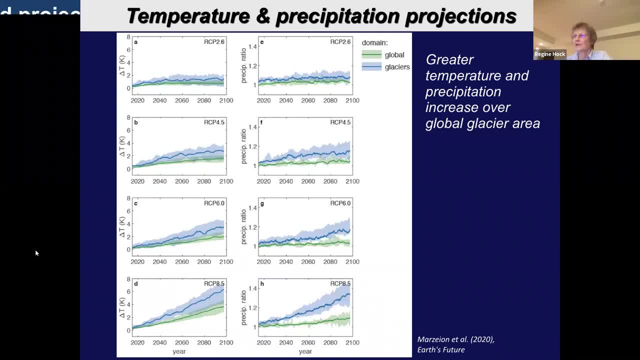 translate into temperature and precipitation changes. what you see here is the time series of temperature and precipitation for the four RCPs, both for global mean temperature and the mean only over the Glaciers, here in blue And just here for RCP 8.5, down here. 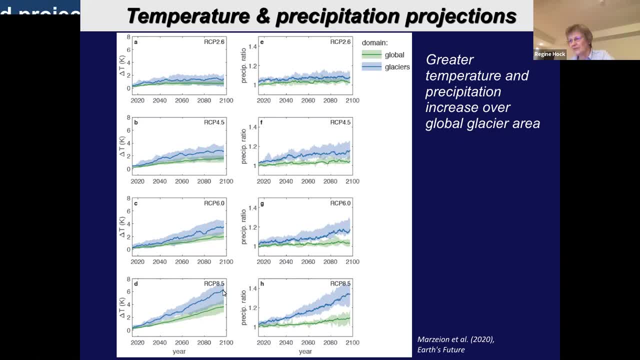 by the end of the century about six degree temperature increase and about a 30% increase in precipitation. And important to note, of course, is that the precipitation, the temperature and precipitation increases are much larger over the global Glacier area. Here you see the result. 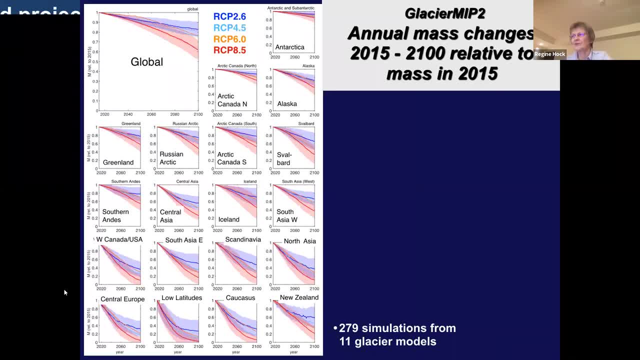 the annual mass changes, again relative to the mass in 2015, for the globe and also for the 19 RGI regions. What you see is the multi-model ensemble median. The shading is plus minus the standard deviation of the ensemble. 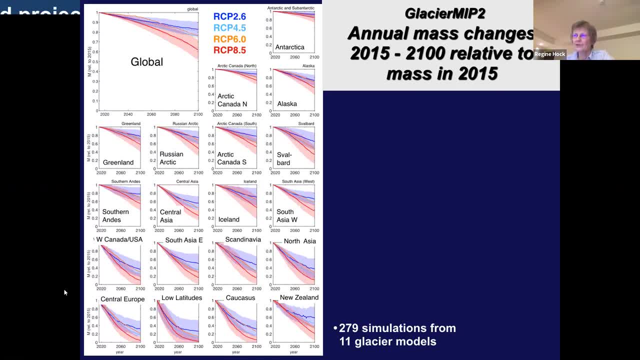 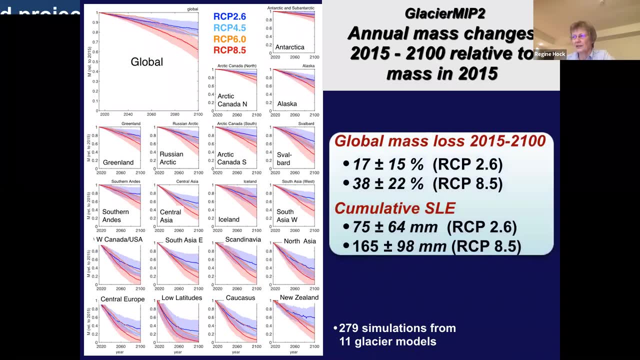 And, but the shading only shown here for two scenarios. for clarity, The global mass losses are here: between 17 and 38% by the end of the century, depending on the RCP scenario and the cumulative sea level equivalent about 75 up to 165 millimeters. 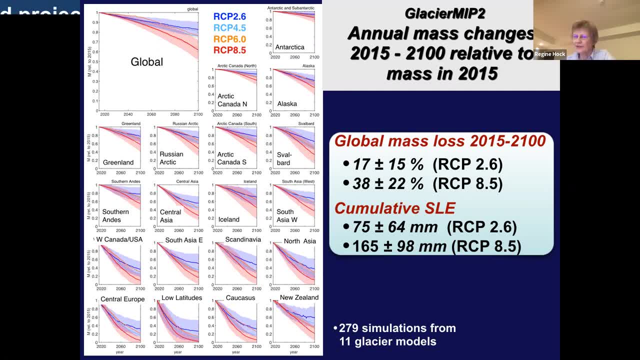 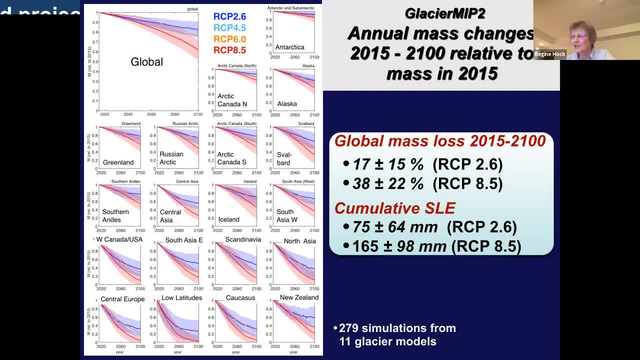 than the previous study, but within the error margins, And that is because two new models were added that had significantly lower sensitivity. The regions here are sorted by relative mass loss And again what we see is the regions- Yeah, with a lot of ice have a lower relative mass losses. 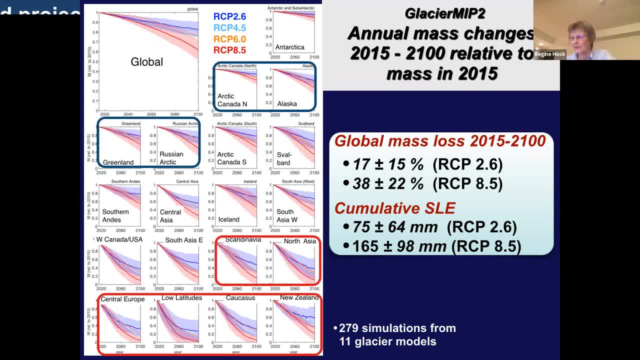 than the regions with with with little ice. We're in some regions that Glaciers are projected to were. in some regions the Glaciers are projected to were. in some regions, the Glaciers are projected to essentially disappear. 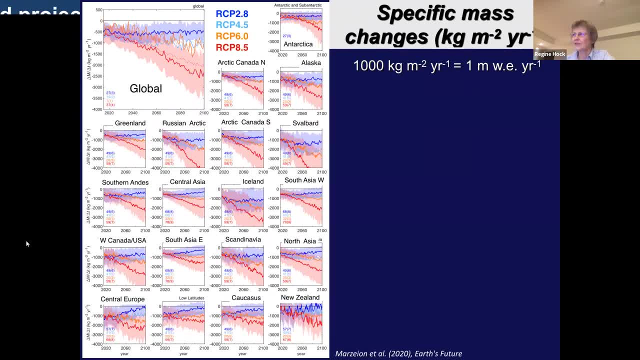 Here are the mass projections in a different unit, In specific mass changes, so in kilograms per square meters per year. this provides a better indicator of the climate conditions that force these laser changes, And a thousand kilograms per square meter is one meter water equivalent. 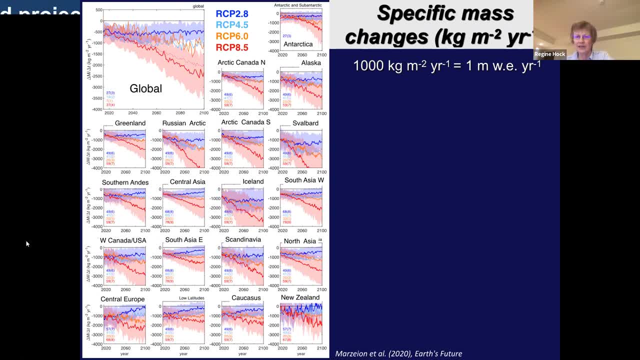 So what is shown here is essentially the average thinning rates in the average over the glacier area for these different regions, in water equivalent, And what you see is that in for RCP 2.6, you don't really see much change for all the regions. 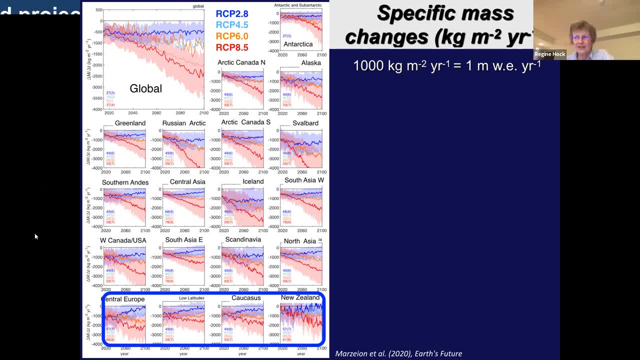 except here, for these regions that are very, very have little ice, like Central Europe or Caucasus, New Zealand, the mass balance becomes less negative with time, So the glaciers essentially reach an equilibrium by the end of the century For RCP 8.5,. this is not the case. 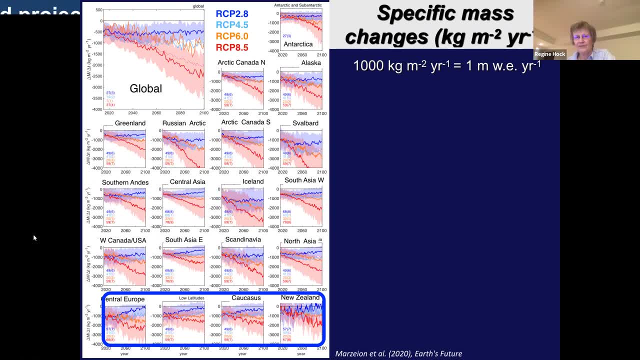 This is much more negative mass balances, increasingly negative mass balances, specific balances throughout the century, in every single region. However, most negative- this is just, I think it's not true- is that the bottom of the ice is a little bit lower and 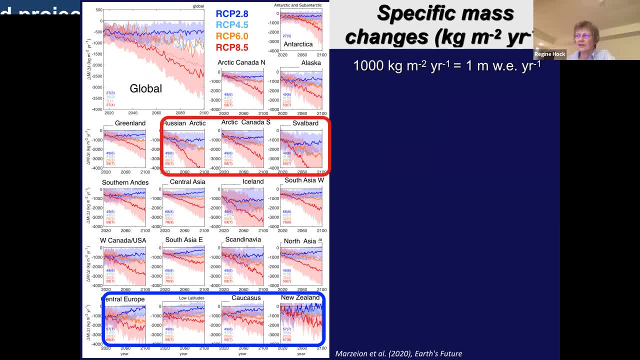 here in the Russian Arctic, Arctic Canada and Svalbard With really extreme values. here Svalbard's off the chart. There's eight meters on average, averaged over all Svalbard, of thinning by the end of the century. 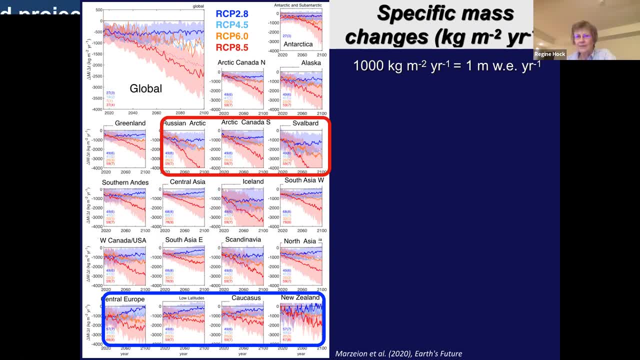 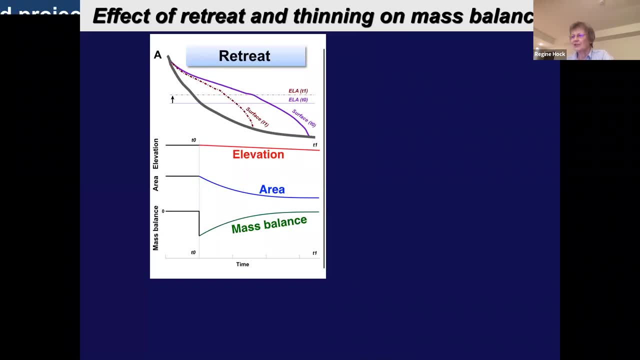 And this is a balance between so of retreat and thinning, And what you see here is to explain these differences. I wanna just go through this here: The effect of a climate step change. there's two opposing feedback mechanisms. First, the retreat effect: when the glacier retreats. 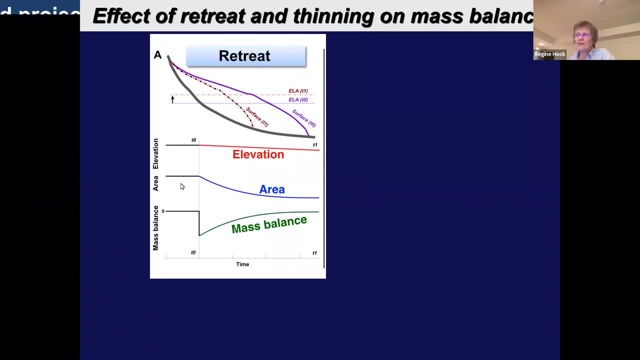 the elevation will go down, but not as much or area will decrease. But as the glacier retreats into a colder climate, it puts itself essentially into a colder local climate, even if the climate doesn't change and the mass balance approach is zero again. 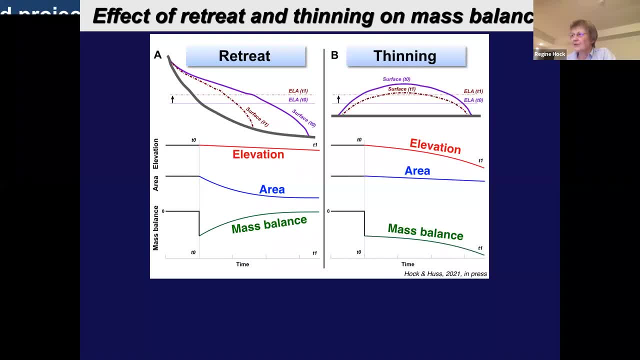 it finds a new equilibrium. But if thinning dominates- typically for ice caps or low-lying large glaciers- the area doesn't change much, but the elevation goes down and then you have a runaway effect, positive feedback and the mass balance. 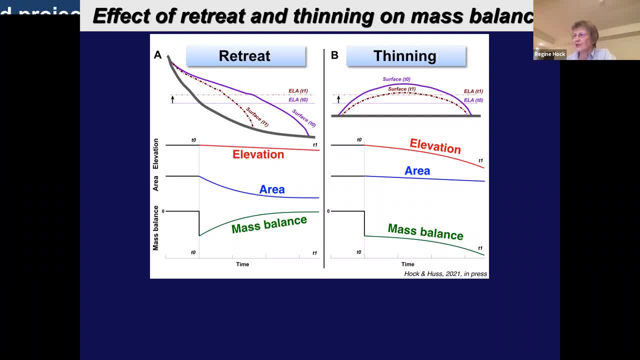 the specific mass balance becomes more and more negative. So essentially, here you have the retreat effect. you always have both effects. The retreat effect is dominating, here It's a stabilizing, a negative feedback. And when thinning dominates, then it's destabilizing a positive feedback. 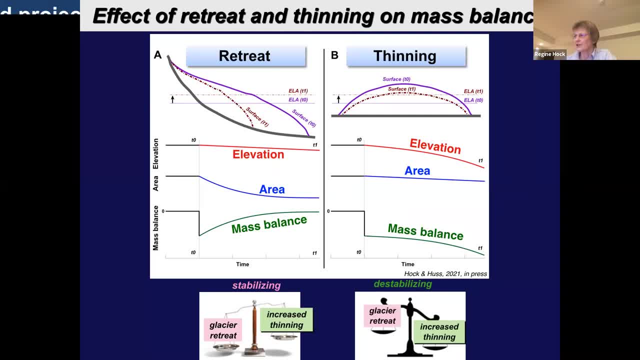 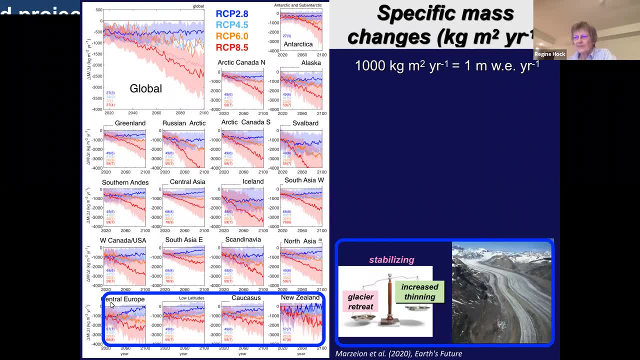 and a totally different time series here for the specific mass balance, And this is exactly what we see here. So for for these regions here in Central Europe and so on, the retreat effect is dominant. Many glaciers will disappear, but those that survive, 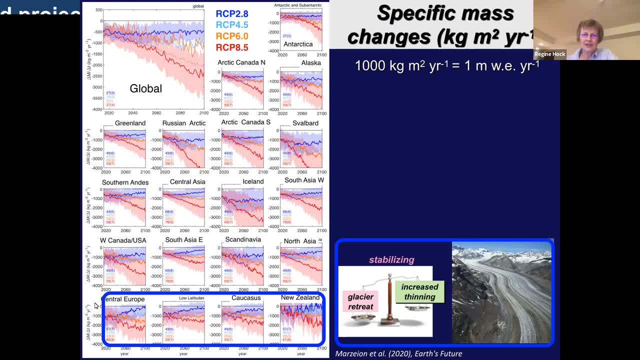 they are able to retreat to colder elevations and reach a new equilibrium For 8.5,. so here the retreat effect is dominant. But for the 8.5 scenario this is not possible. The warming is way too intense. It's not possible to compensate. 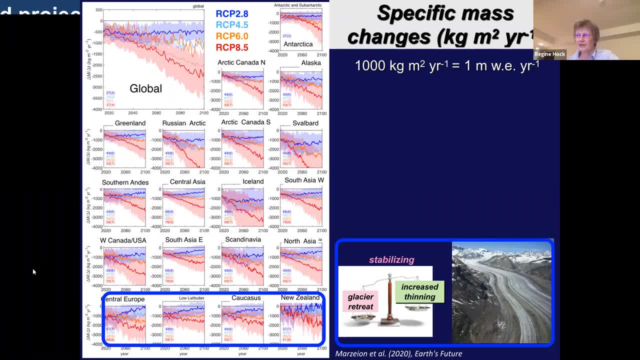 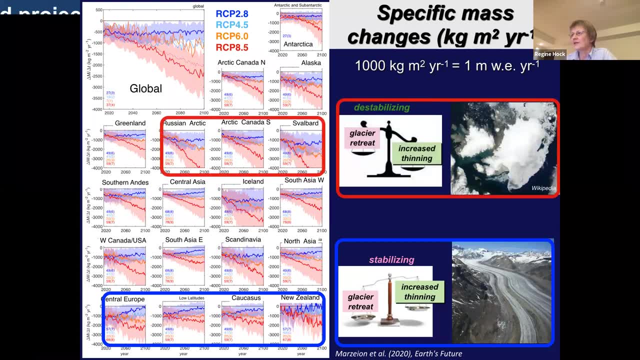 so that the retreat effect cannot compensate for these increases in temperature. And why here? for these regions in Arctic, Canada and Russian Arctic, there's a lot of ice caps, So that's where the thinning effect is dominating, And this is what really drives these much. 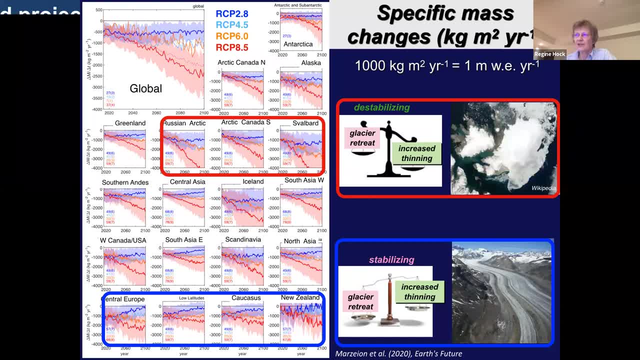 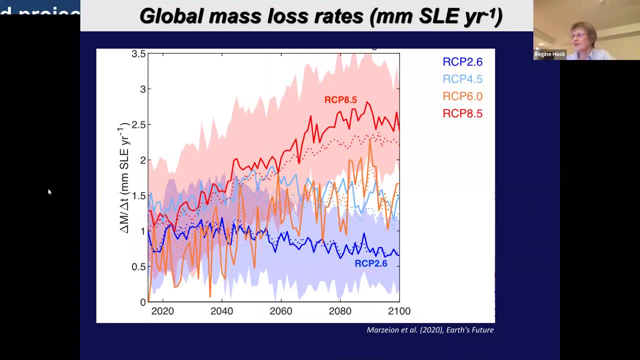 much larger specific mass loss rates in these regions, here In these polar regions, compared to the other regions. And again, projections in yet another unit, this time in millimeter sea level equivalent. What you see is either for RCP 2.6,. 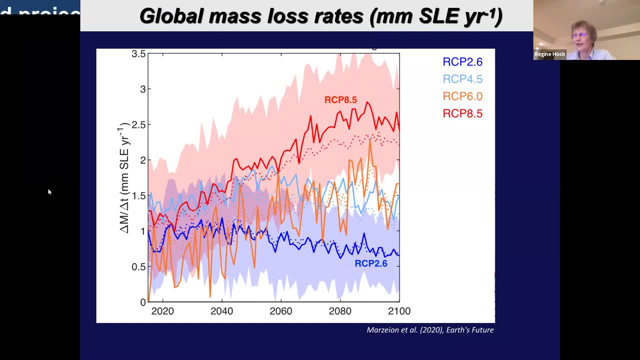 there's a little bit of an increase, but then sea level will actually decrease slowly over time. So here again, the warming is only moderate. Many glaciers- I mean many- will disappear, but those that survive retreat to colder, higher elevations. 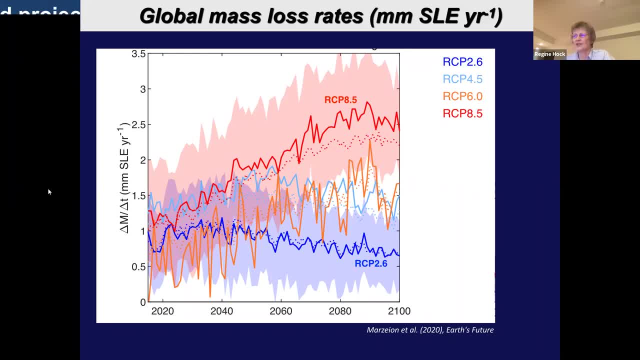 And the mass loss from these glaciers is going down. Whereas for RCP 8.5, there's a steady increase until close to the end of the century, The warming is too strong to compensate, so that the retreat effect cannot compensate for that. 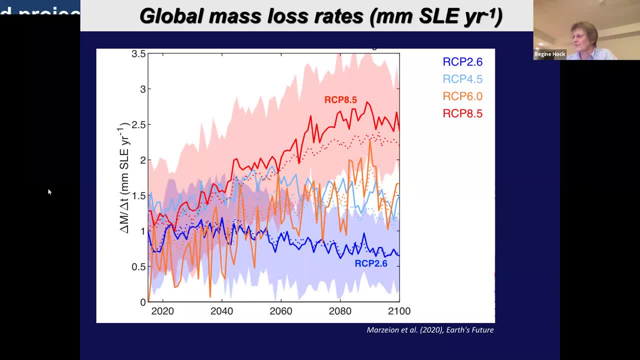 and the rates go up and up until the end of the century. What is also notable is that the sea level contributions here by the end of the century from the lasers for the RCP 8.5, the mean is here 2.5 millimeters. 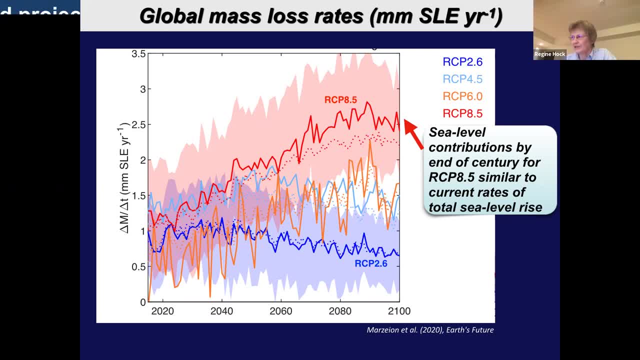 and some of the simulations go up to 3.5 millimeters per year. So that corresponds to the current rates of total sea level rise. Sea level rise at the current rate is about three to 3.5 and three millimeters per year. 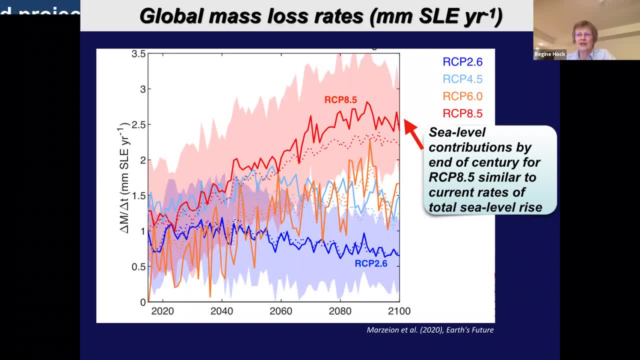 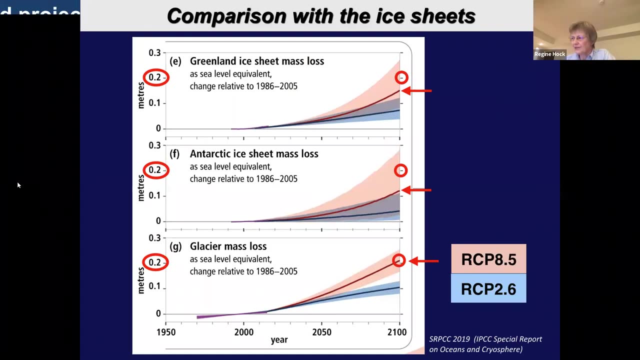 And what we project here by the end of the century is that the glaciers will contribute just as much to sea level, like the entire sea level rise rate that we have right now. The next slide shows a comparison with the ice sheets From the IPCC, the recent special report. 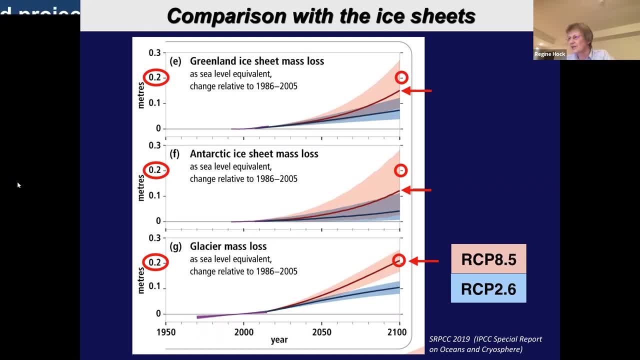 on the oceans and the cryosphere, And what you see here is maybe something that you wouldn't expect, but that by the end of the century, the simulations here from this report shows that the mass losses- the sea level equivalent by the end of the century- is larger than here. the mean 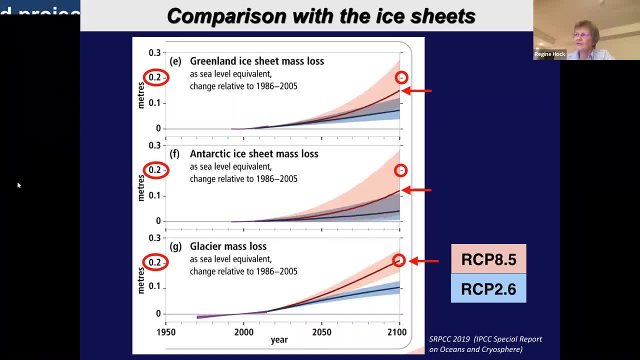 what is projected for Antarctica and Greenland. Of course, here for the ice sheets, the uncertainties are higher And also it does not include any potential catastrophic collapses In Antarctica, But nevertheless this really shows that for the next until the end of the century, the glaciers are really 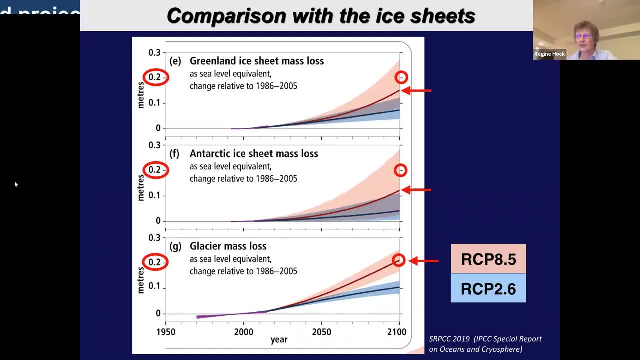 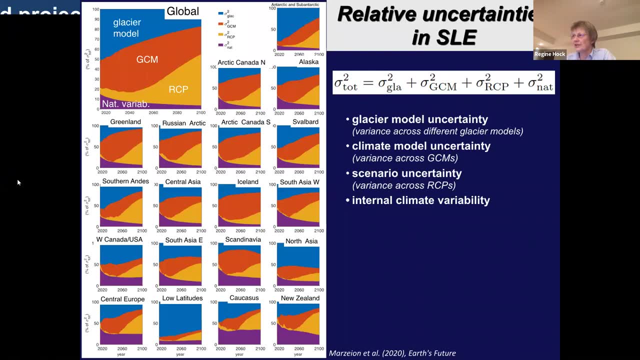 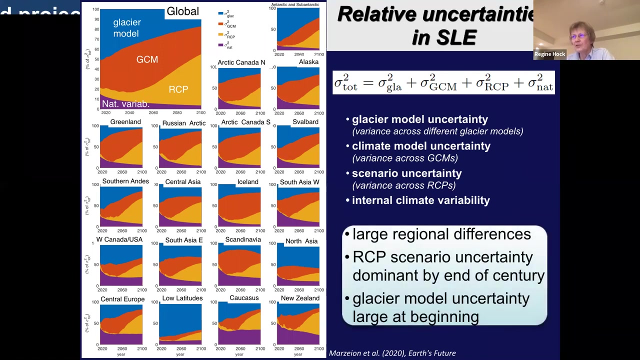 a major, continue to be a major contributor to sea level rise. Here looked at the relative uncertainties in these projections, So the uncertainties here the assumption is that the uncertainties due to the possibility of the rising sea level rise is the most likely to occur. 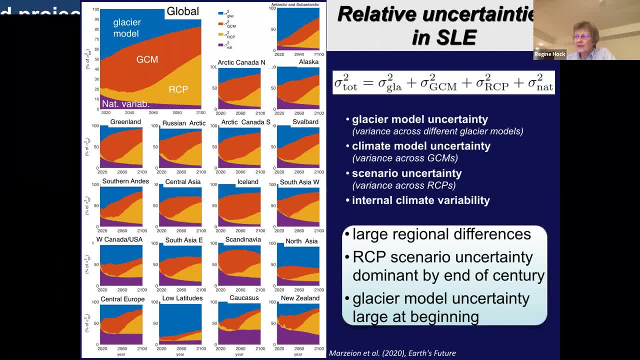 And that's because the recent data from the ESA data, from the NASA data, is showing that the ocean levels and the sea level rise are not very high. They're not very high that the glacier model uncertainty is actually quite large in the beginning. so in the first few 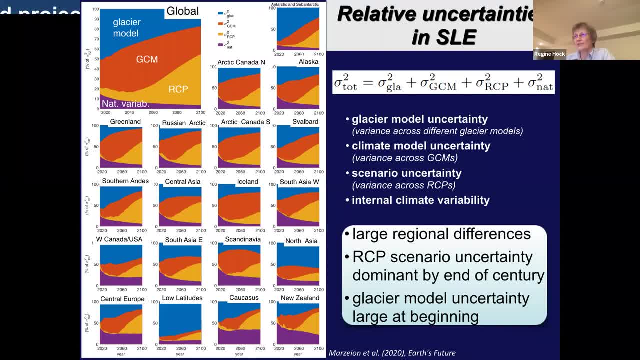 decades. it's really um in many regions and also globally are a large contribution by the glacier model. so that also means that improving the glacier models can really in reduce the uncertainty in the next decades to come. so this really helps us analysis to to see where to reduce. 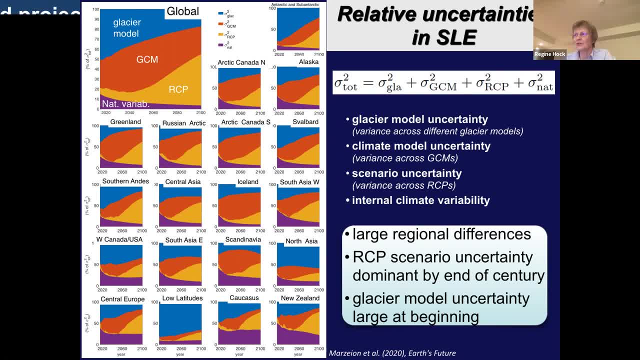 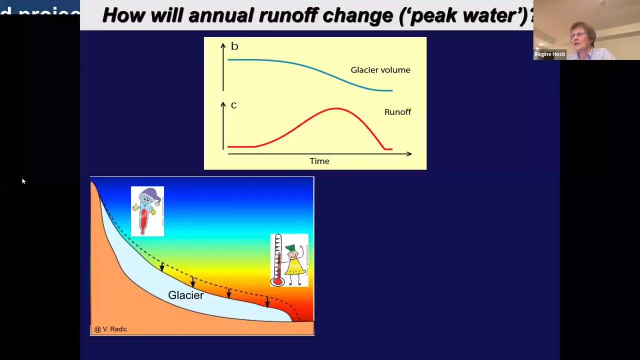 where we benefit most in when we try to reduce the uncertainties. um, this was a lot about sea level, but of course the glacier changes impact, like water resources, runoff, and i want to spend a few minutes now how glacier these mass changes affect runoff. so, first of all, how will annual runoff change when the glaciers retreat? 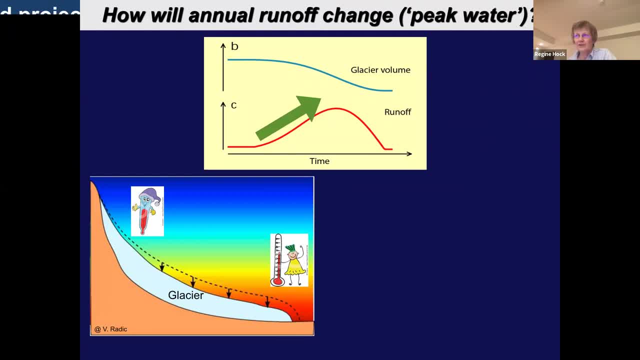 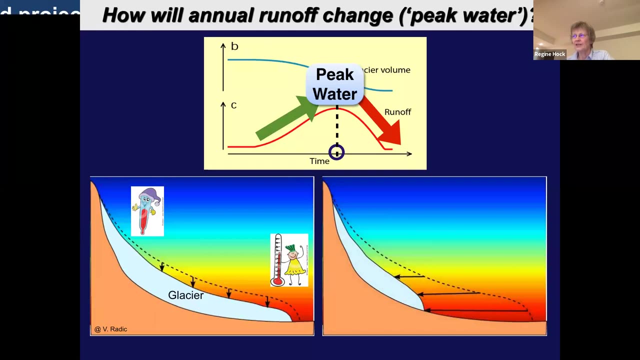 um, first, typically runoff annual runoff goes up, and it can go up by like 50, 60 percent, quite substantial. and as the glaciers then retreat further, uh, the runoff goes down, and so somewhere there's a turning point, what we call peak water, and the timing of peak water is of course important. 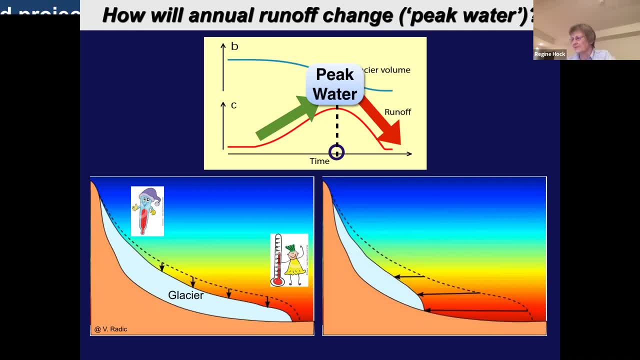 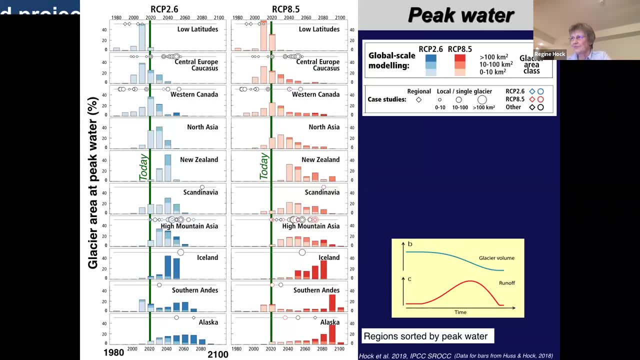 to know for water resources management. so so what you see here is a compilation of peak water for different regions in the world from the ipcc s-rock report. regions are sorted by peak water and this is really a compilation of hundreds of studies in the, in the literature and the bars are based on. 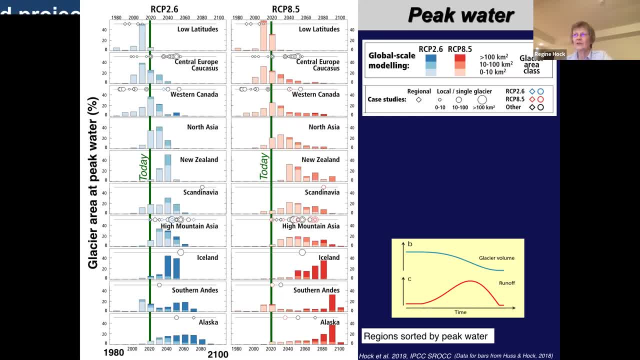 a modeling study? um modeling every single glacier in the world and when peak water is, and the each bar shows how much? um- because there's of course variations within a region- how many percent of a region? um has reached peak water at a certain time. so, for instance, here for the low latitudes, about 50 of p? uh. the area reaches peak water by 2010, so that's. 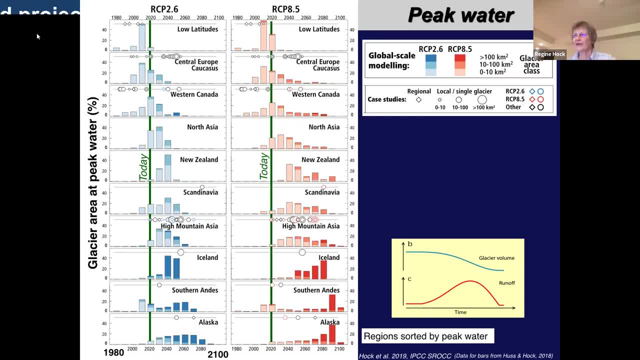 what these bars mean. so they add up to a hundred percent of area and what? what you see is, um, that peak water in the regions with little eyes. um, peak water has already been reached in the low latitudes. that means it's on the down slope here. runoff will go down in the future in regions with. 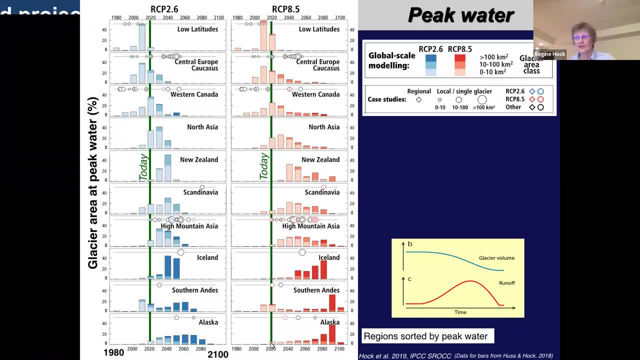 a lot of ice, um like here. alaska peak water has not been uh reached and and just reached in a few of the area, but it will be reaching the future and most of the area will will reach it at the towards the end of the century. you also see like high mountain asia, for instance. the peak is like 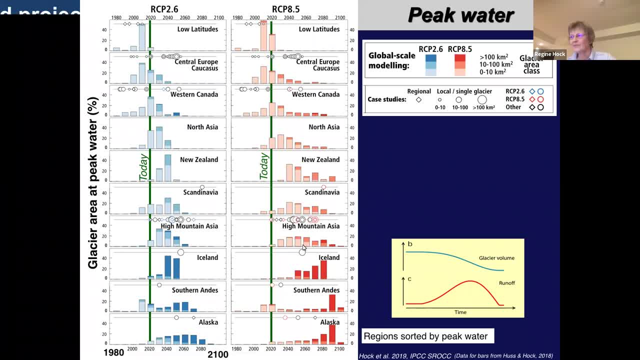 most of the regions here reach it by 2050, but it's widespread. depending where you are um, the different colors show the size of the glaciers and you also see here that the glaciers are that are larger, which are uh reach peak water later than than the smaller glaciers. for rcp 2.6. 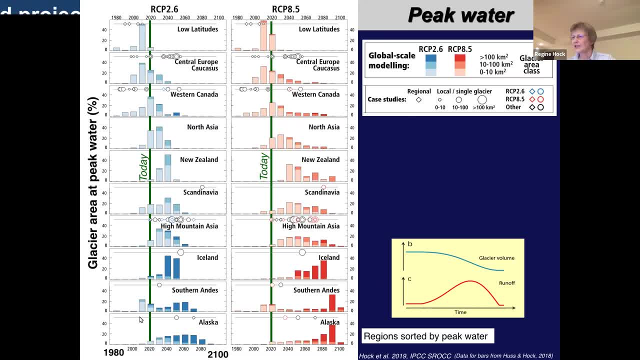 peak water is generally reached earlier, and that makes sense. it's simply because under this more moderate scenario, the, the peak water, reaches earlier than the smaller glaciers. many glaciers are approaching new equilibrium. that means then the runoff goes down again, because then as less mass is discharged, but for rcp 8.5, the, the melt is more and more intensified. 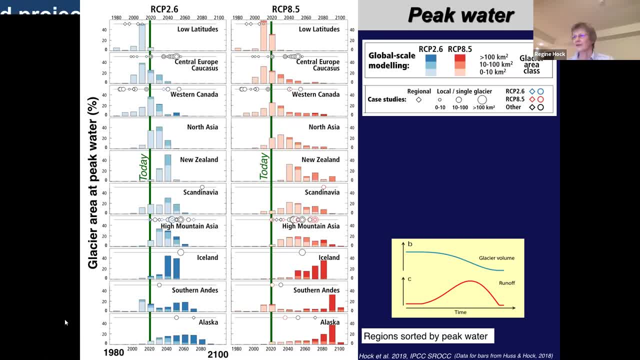 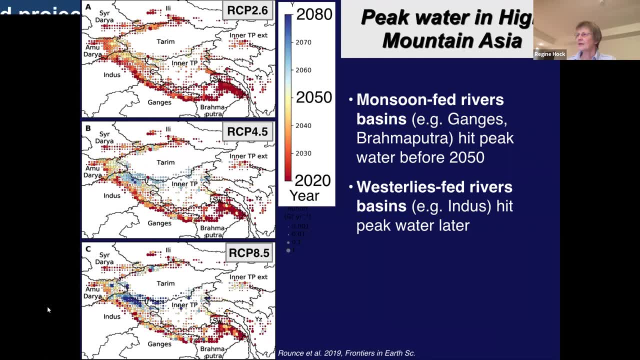 and peak water is reached much later. the next slide- yeah, let's just summarize here. the next slide- shows just an example of a more detailed study here by david rounds, also calculating peak water for every single glacier here in high mountain asia, and what you see is a very differentiated picture here. overall, the pattern is similar for all rcps. 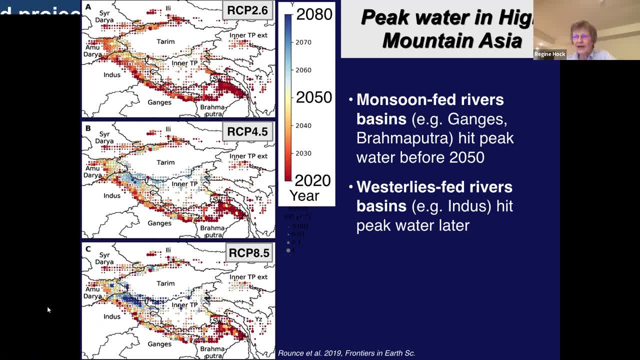 but the spatial variations are more pronounced for higher rcps. so the colors of the year of peak water, like blue- it's reached at the end of the century- and dark red- uh, essentially now has already been reached and we see here large spatial variations within the same region. 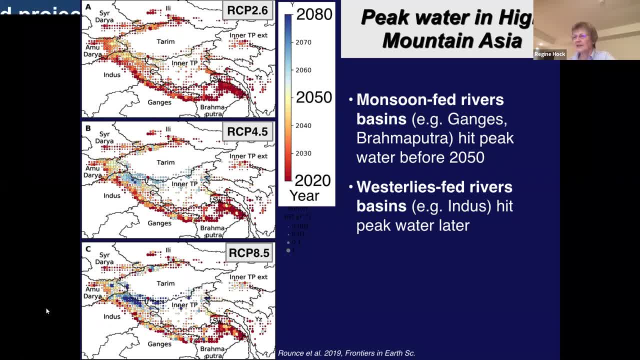 the regions that are monsoon fed here- these are like the gangas and brahmaputra down here- have reached already peak water or about to hit it latest by 2050, whereas the basins like the indus here that are fed by the westerlies, they hit peak water much later. but even here within the basin, 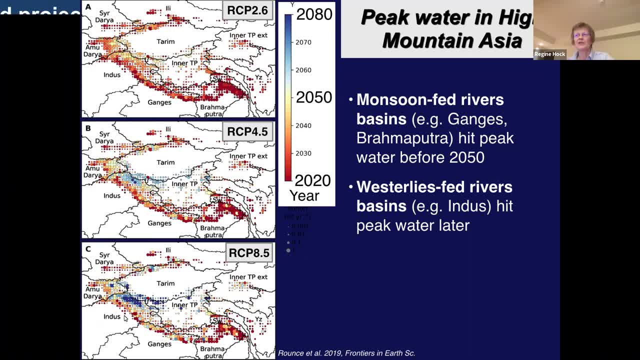 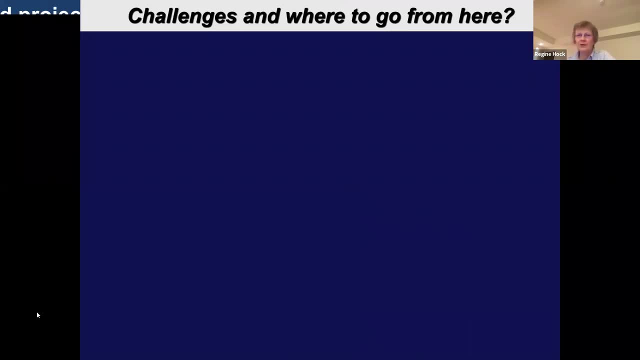 there's huge spatial variations within on a very, very small scale, and that's, of course, important for our on a local scale for water resources. okay, so what are the challenges in global, global projections and where do we go from here? um, most models compute mass change of every single glacier individually, and this is, of course, i mean. 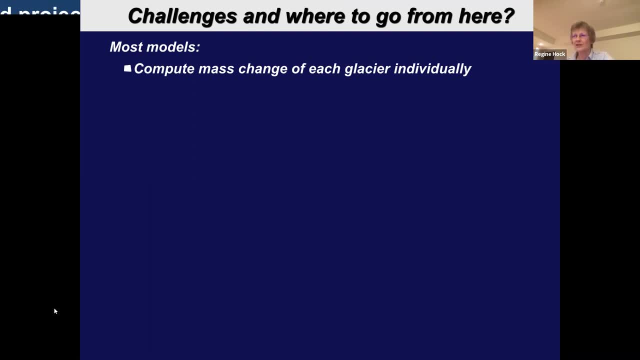 quite sophisticated and great, but most models are still very, very simple um the climate forcing. all of them use all but two. use just temperature and precipitation. um, often just monthly mean. um, most of them are simple degree day models. uh, most of them use some scaling or a simple geo geometric model to to model the geometric 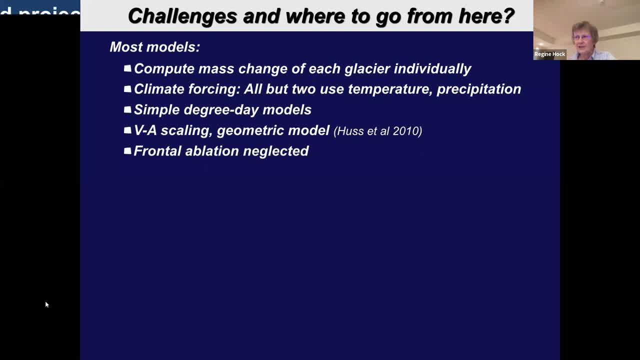 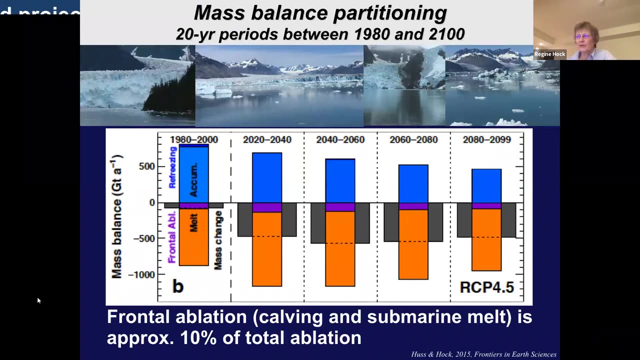 changes. um frontal ablation is neglected, um so the calving and submarine melt neglected by all but one model, and that one model has shown that. uh, it accounts approximately for 10 percent of total ablation. so what you see here is the model, the projection, different time periods um total melt and total accumulation. 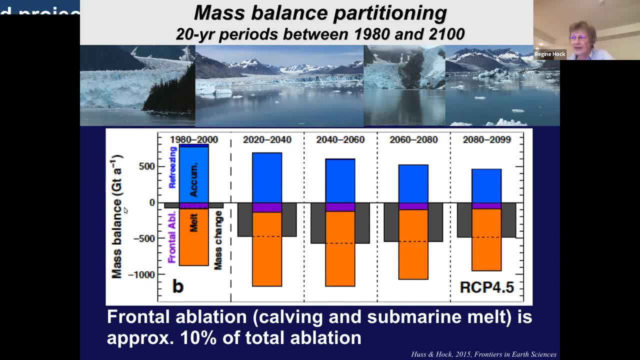 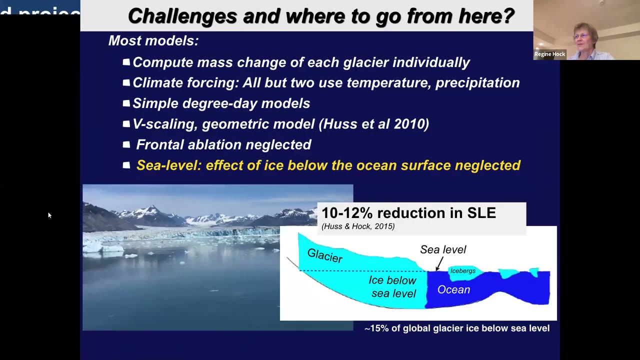 and then here in purple you see the frontal ablation and gray is the net net balance. so in the important is of course 10 percent um. it's systematic, it's always a mass loss and this is really the only model in the literature that includes frontal ablation um about 15 of the global. 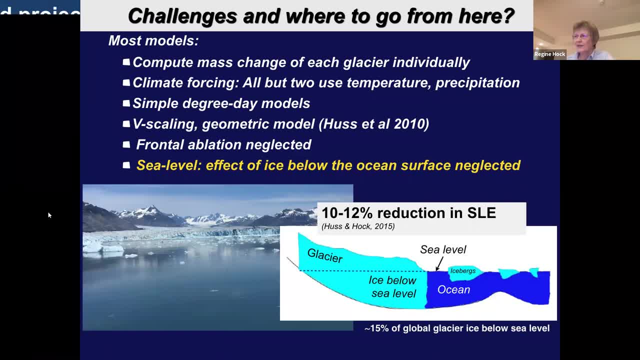 glacier area is below sea level and that effect has also only been uh taken into account by one model, which has shown that it's a 10 to 12 percent decrease in the total ablation rate, and then the other model, which has shown that it's a 10 to 12 percent reduction in sea level. if you 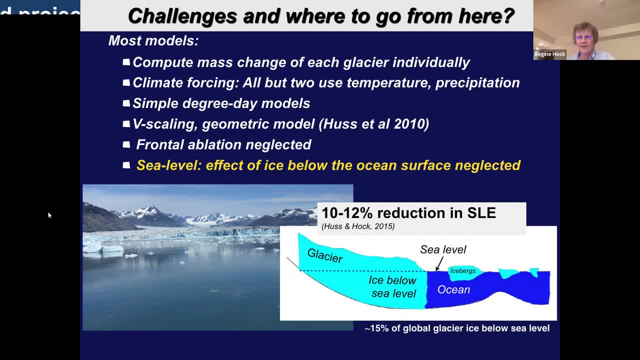 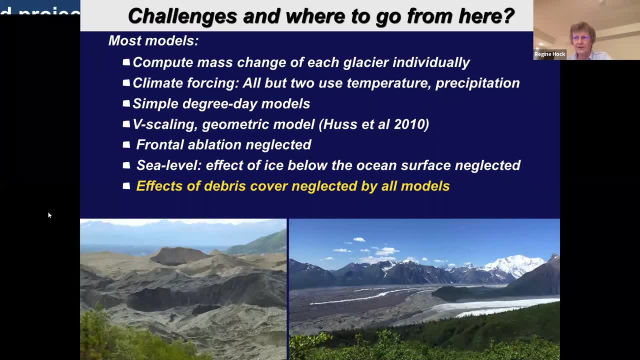 account for that ice that is already displacing or ocean water. then the effects of debris cover are neglected by all models, uh that are published in the literature, and about four to seven percent of global lasers are covered by debris and potentially suppressing melt. and then all models suffer from over. 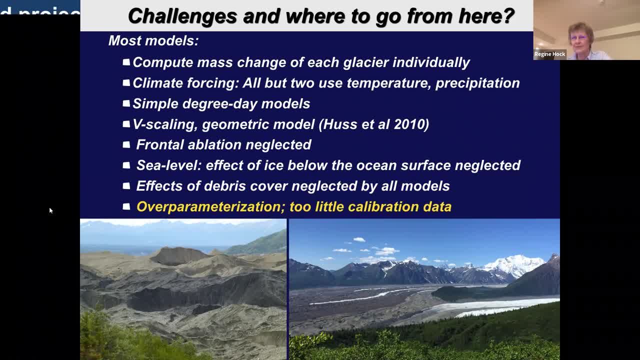 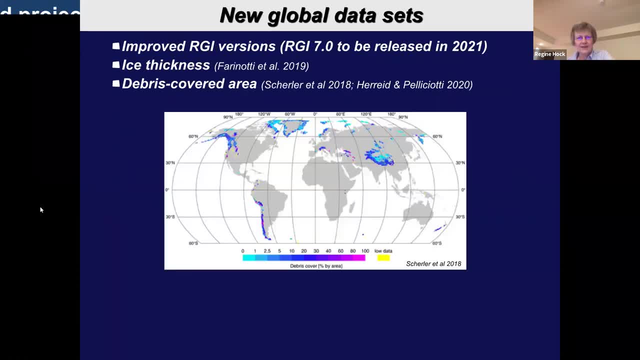 15 percent of global ice, and so there is a lot of concern about the potential of these models because they are very, very rare and there is too little calibration data to really constrain the model parameters that all these models have- to constrain them well. but there's really good news for future modeling efforts: there's more, more large-scale data. 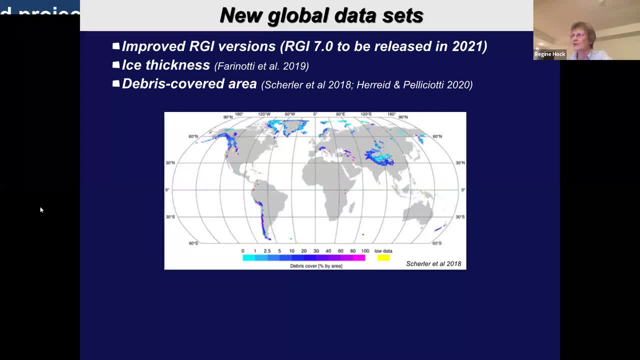 sets emerging that are available for initializing and for calibrating the models more accurately. there's improved rgi versions, a new version coming out, new global scale ice thickness estimate. There we now have maps of the debris cover around the world, two different estimates here. 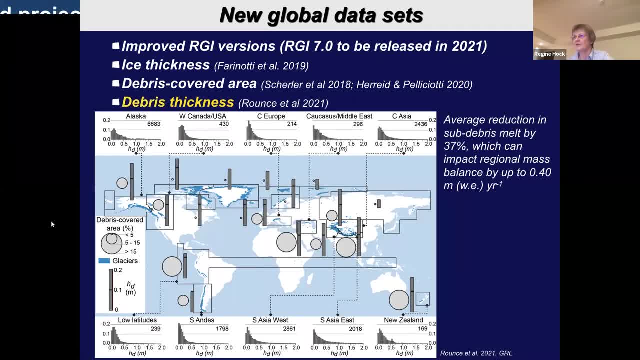 And not quite yet published here by David Rounds new map of debris thickness of every single glacier in the world. So what you see here in the circles show the debris cover the area and the bars show the debris thickness- A median thickness of 15 centimeters across the world. 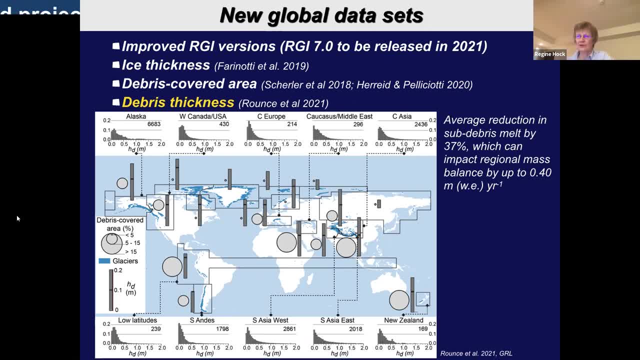 And the big question is, of course: does it matter if only four to 7% globally are covered by debris? And here his simulations show that there's an average reduction in sub-debris melt by 37%, And it does impact regional mass balances in some regions. 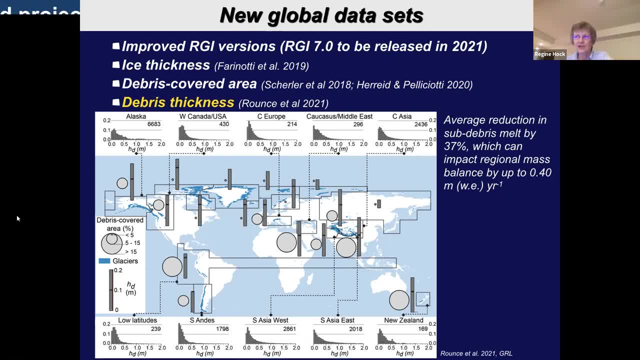 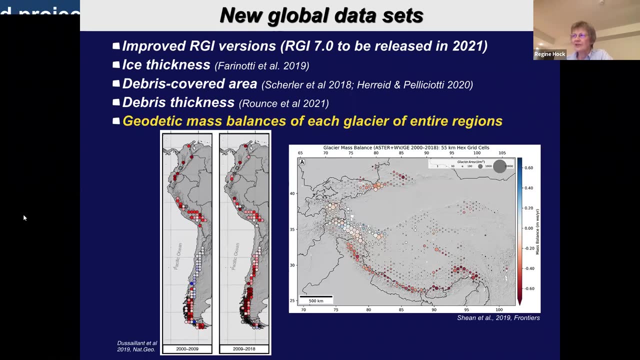 and up to 40 centimeters, So that's substantial, and it's really important to include debris cover into these simulations. Another good news is that geodetic balances are available now for every single glacier of entire regions, And that is an especially important. 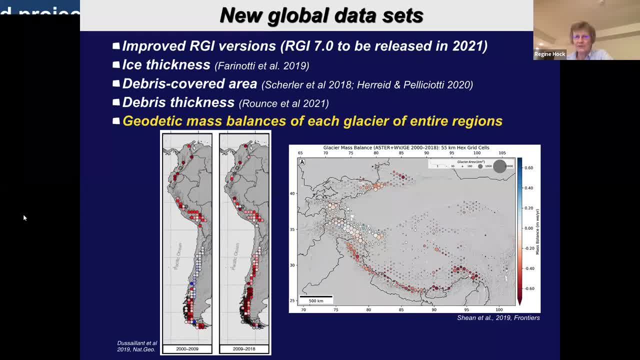 for calibrating the mass balance models, And this is, of course, a huge step compared to like just 15 years ago, or less than that, where we only had a few glaciers from the WGMS to do our calibrations with, So only 15 years ago. 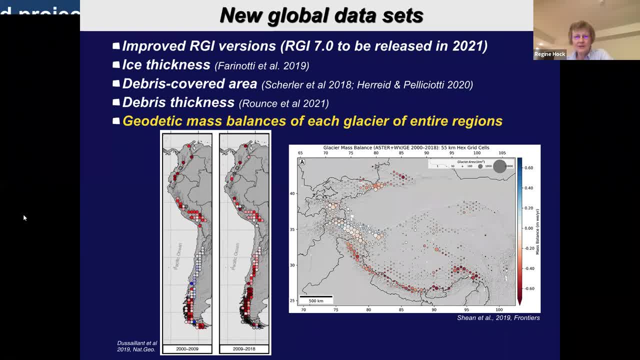 we had very little incomplete data, incomplete inventory. Global projections were based on calibrating a few measured glaciers in the world. So the progress in really the last just a bit more than a decade, it's just enormous. We now have large scale satellite-derived global data sets. 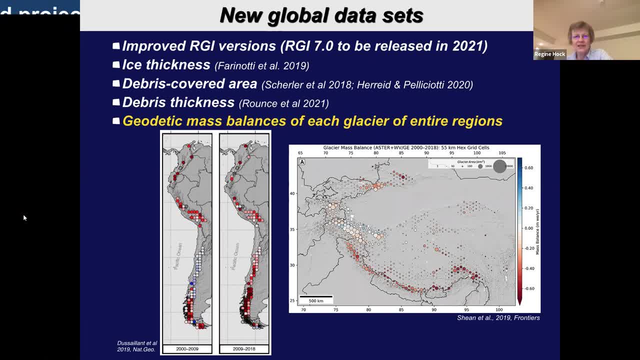 that are publicly available And that allow us to initialize and calibrate and evaluate our models with really unprecedented accuracy. It's really something like just 15 years ago we could only dream of. So it's also important that is that the global scale. 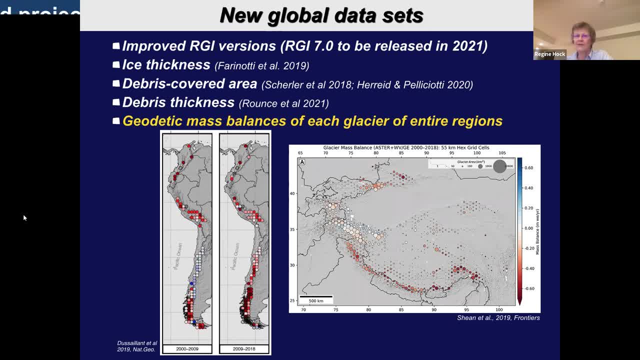 of glacier community has increasingly organized itself in coordinated research efforts like the RGI Working Group, the RACMEC Working Group, Glacier, MIP and those international initiatives have really been essential in making such great, great progress. So the future is really bright. 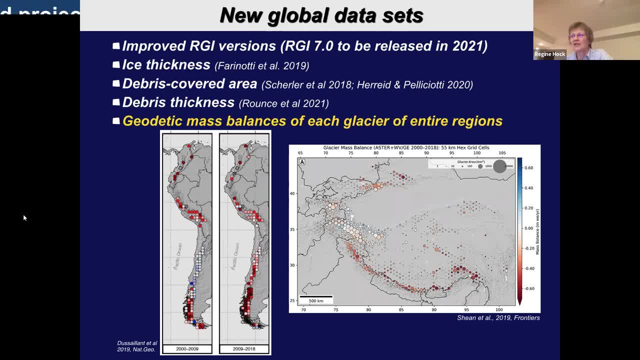 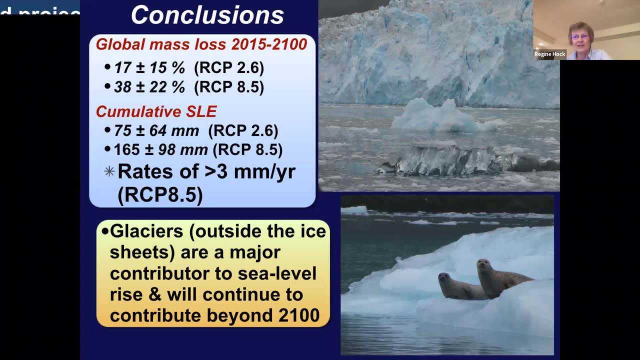 And I think there's really a lot more to come with all these new data sets. It's really unprecedented opportunities. we have to reduce the uncertainties in these projections. And yeah, here are just some conclusions, some numbers and general conclusion, and I leave you with that. 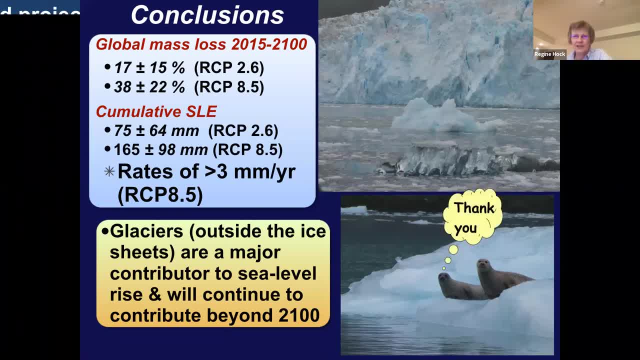 And thank you very much for your attention And I'm happy to take any questions. Thank you very much, Indeed, Regina. we've already got a couple of questions on the chat, but if people want to type into the chat, if they'd like to ask a question, and anyone on Facebook too, 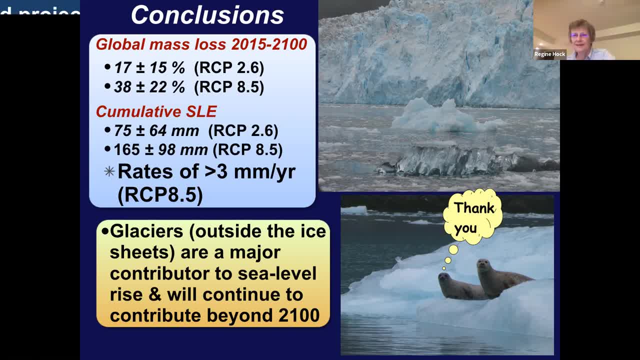 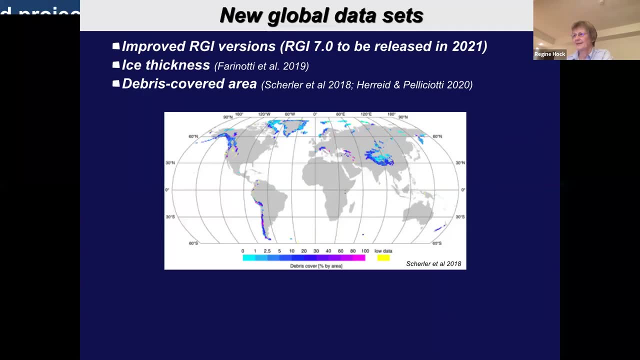 So we start off with a question from Sasha Leidman. Do you want to unmute yourself and ask a question, Sasha? Yeah, I was just confused, looking at that graph of the different peak times, about why the Alaska and the Western Canada. 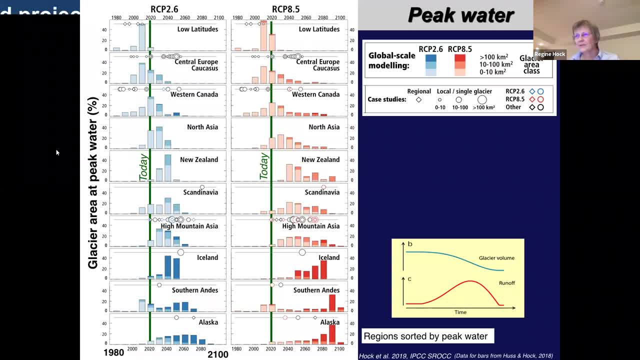 would be so different. That is because in Western Canada it's actually quite a lot of ice there, but it's small majors, It's small valley majors, And in Alaska you have these gigantic ice fields and ice caps that continue to lose mass. 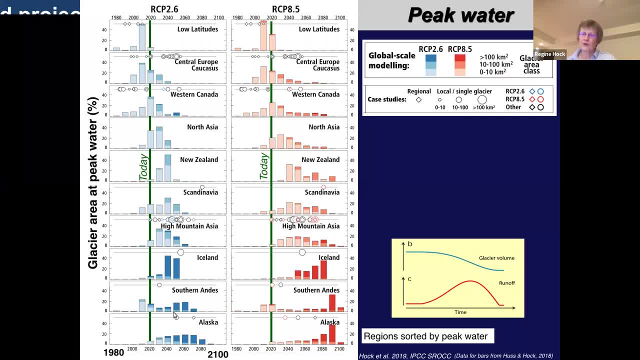 And that's why peak water is so important. Yeah, But it's much, much later. OK, thank you. There's a question on Facebook from Berta Gonzalez-Sanchez which says: first of all: it says: big thanks for the seminar. 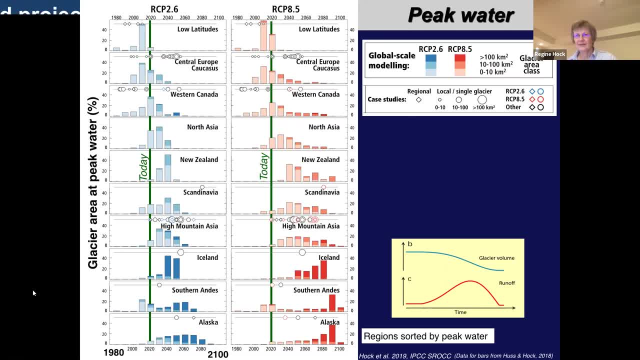 But it also says: maybe you said at the beginning or is it included in one of the parameters of the models, but is the effect of albedo included? Yes and no? No, I mean most models have a temperature index, a degree-day model. 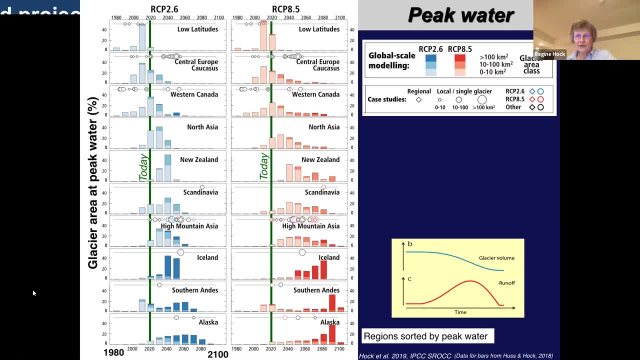 And most models use a different degree-day factor for snow and ice. So they model the snow cover and then the snow cover is eliminated. Then you use the degree-day factor for ice, which is larger, And that is, of course, the different degree-day factors. 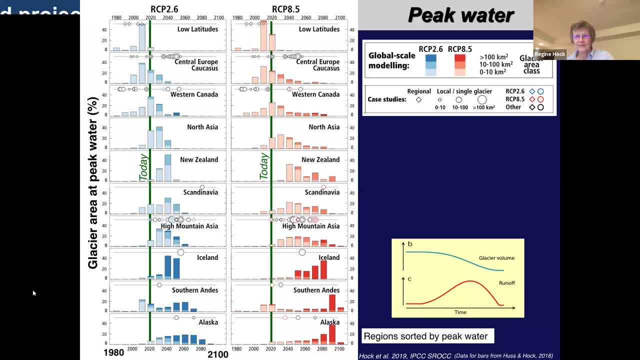 The idea is to account for albedo. OK, thank you, Ben Redmond-Rosch. do you want to ask your question? Hi Rajin, Thanks for the great talk. My question was also regarding the albedo and the material. 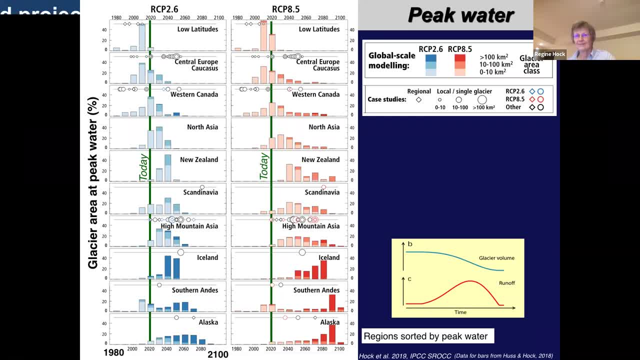 covering the glaciers, Just regarding whether it's just the boulders and the rock material or whether it's also things like black carbon, dust and aerosols which are also to be considered in the models. Yes, I mean, it definitely affects. 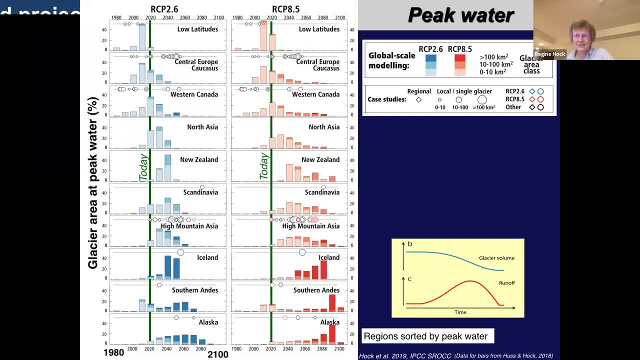 The mass balance, but it's not considered in the models, And that is another thing that, yeah, for the future it's not considered. Thank you, Steve Warren. Oh, yes, Regina, Fairly early in your talk you showed. 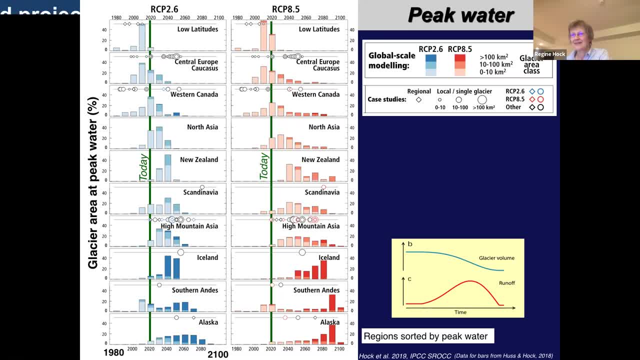 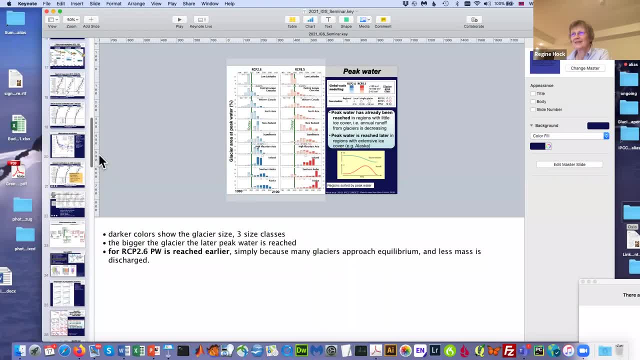 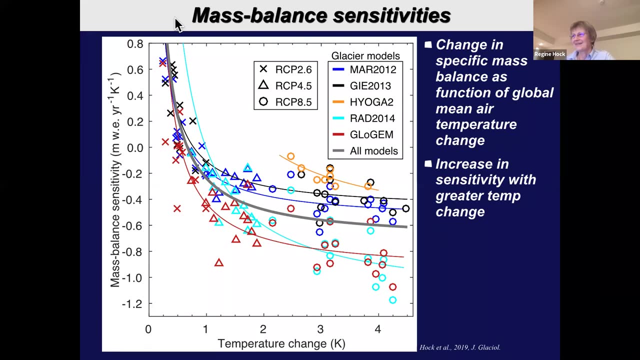 a plot of the sensitivity of mass balance to temperature change, And there was a transition from positive to negative, And so I wondered, I wanted to ask, if you could say something more about that. that it's like less than half a degree temperature change. 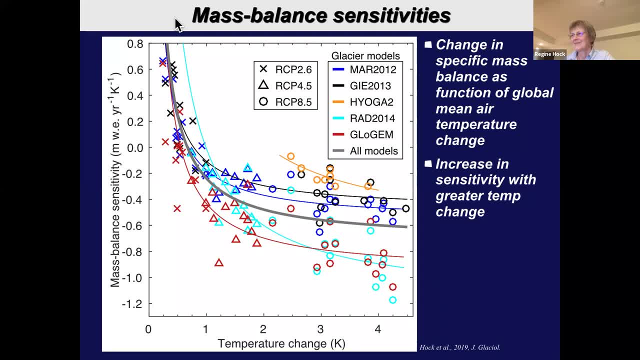 The sensitivity is positive and then it goes to negative. Yes, I remember that when we found that we had a great explanation, I just forgot about it. It might also be just the uncertainty in light. It's like the temperature change. 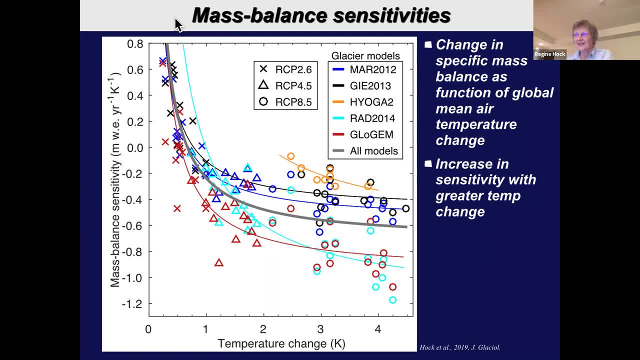 I mean you extract it from the GCMs. So I would say this is not real, This is just sort of. And then the other thing is, of course it's not only the temperature change, because there's also precipitation changes. 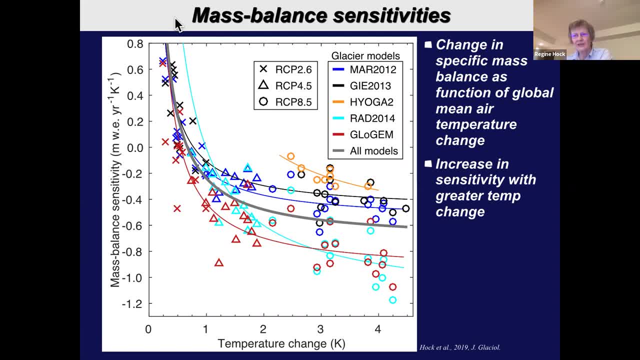 And then when you only have a little bit of a temperature change, yeah, that's it. If you only have a little bit of a temperature change, then if there's also a precipitation change, then it messes up your sensitivity here. OK. 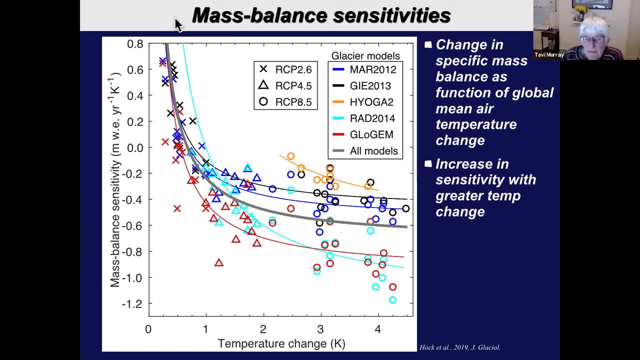 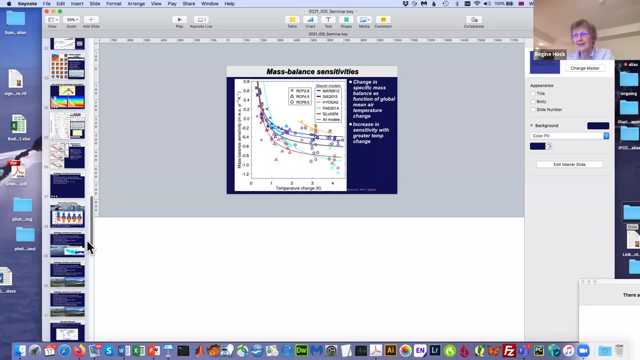 So, Adam, Adam, Yes, yes, I'm here And my question it's about output and different model about Russian Arctic. What problem? A lot of ice cap and you have a different model for ice cap. Why different output? Different model? yeah, different model. 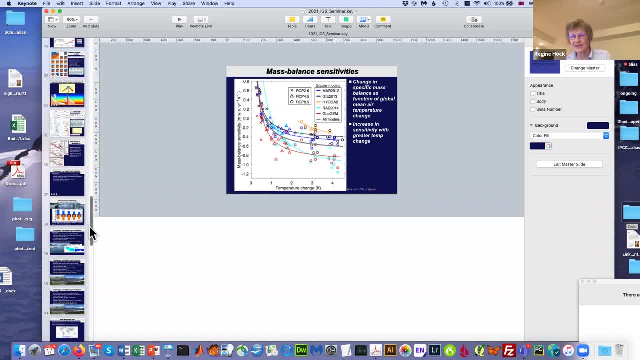 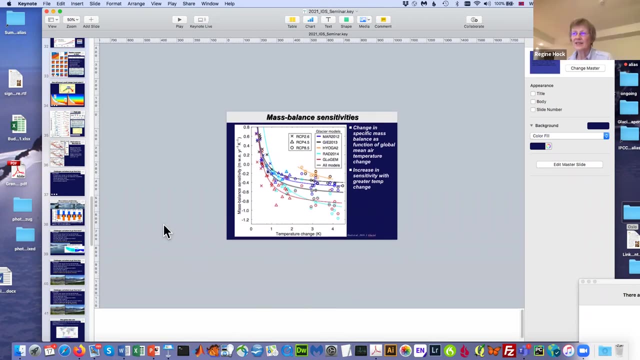 You mean, if we have a different model for the ice caps- Yes, yes, because it's output- and different for forecasting for Russian Arctic? I don't see. Yes, I mean it's not a different model. You run essentially the same model. 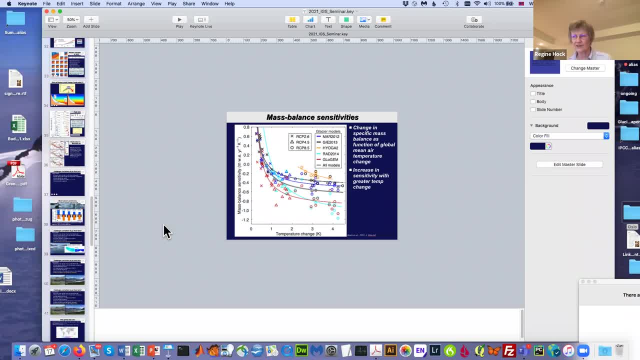 which is just depending on which model it is. But it can be an elevation-dependent model that just calculates the mass balance for every elevation, And if it's an ice cap or an ice or a glacier, the model doesn't know and it doesn't really matter. 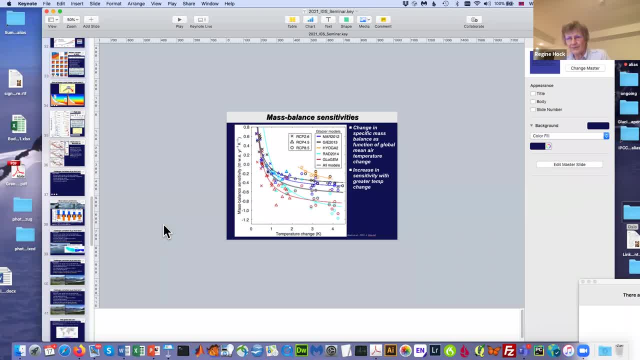 But the different response is only that the ice cap starts thinning and then it puts itself into a warmer climate, and that amplifies then the response to the warming, Whereas the glaciers- and because we have a geometric model in there- when the glaciers retreat. 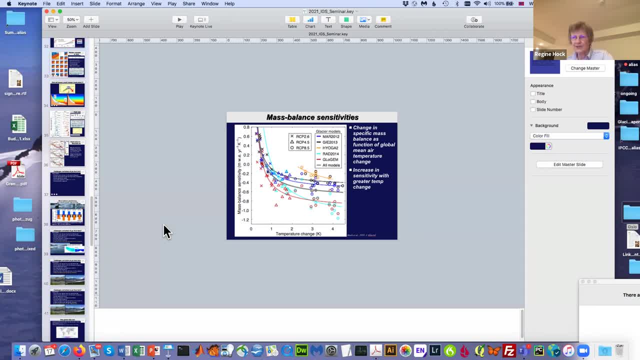 that is accounted for. Then they put themselves into a colder climate And that gets the different responses between the ice caps and the valley glaciers. Thank you so much. Very, very interesting, Great talk. Thank you, Pete Nino. Sorry, couldn't find my microphone. 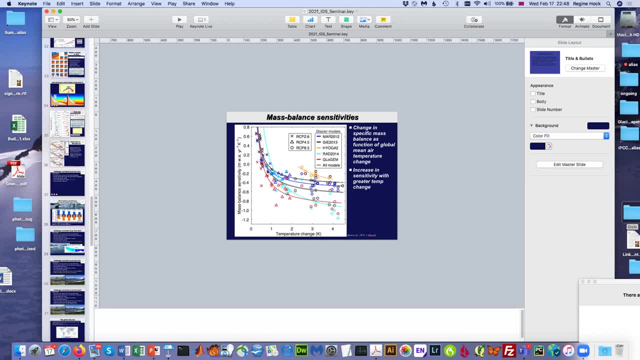 Hi Regina, thanks for that. Hi, You touched on the photo fact that basically just one of the models takes into account frontal ablation of glasses terminating in the ocean. So is it, am I right, that none of them have any sort of dynamic? 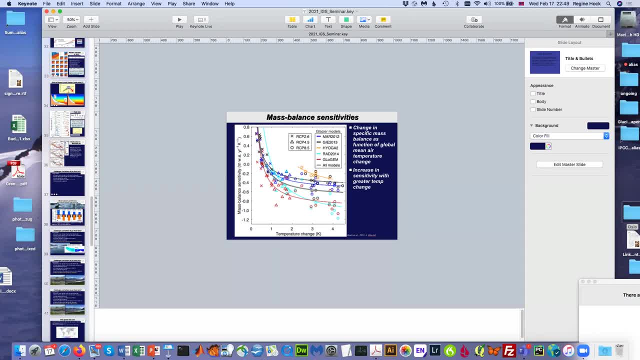 component in terms of they don't take into account how Russian Arctic ice caps, for example, might accelerate or as a result of sort of marine influences. They don't. none of the models do that. It's just surface mass balance. It's just surface mass balance. There's two. 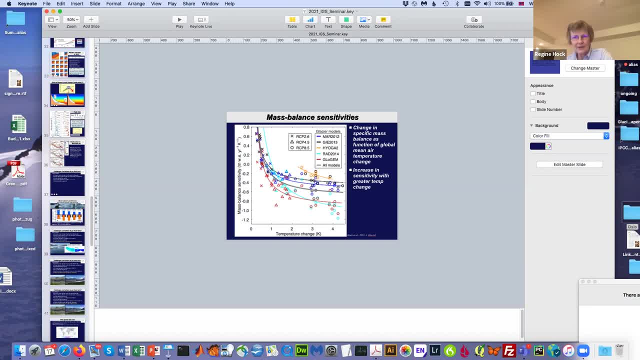 of them are models in the last round that have a simple flow line model in there. But yeah, I mean any acceleration due to some ocean processes is not included. Okay, So is there ever any sort of suggestion of chucking on an extra error margin to account? 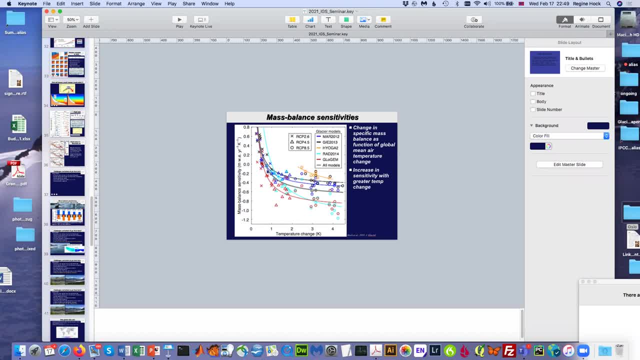 for any acceleration, Because presumably what you're really doing is obviously you've still got error bars, but it's almost like only from one aspect. Yeah, I would say that the frontal ablation is really that's the next big step that we 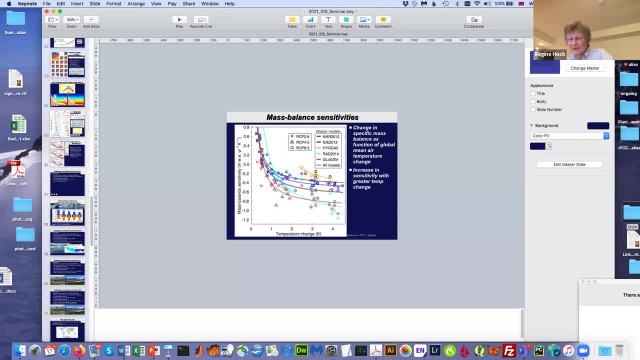 need to tackle because it's systematic And I mean there are some models are now adding modules to compute that, but it's still pretty simple And the big problem is like how to calibrate any parameters And we are hoping- I know there is efforts underway- to actually 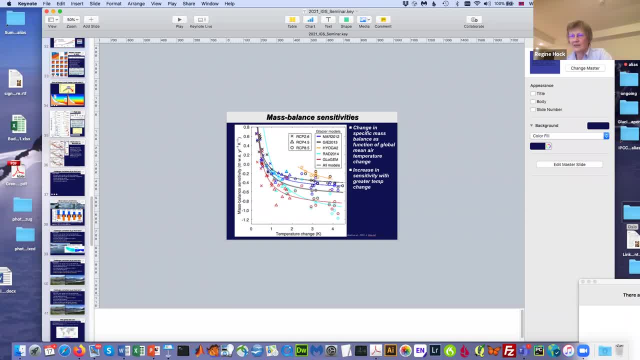 have a lot more like thousands of lasers in the world, But I don't think there's any data that we could use to to reasonably really calibrate any model that we come up with. But this is really sort of the next step And the data is coming out, I think. 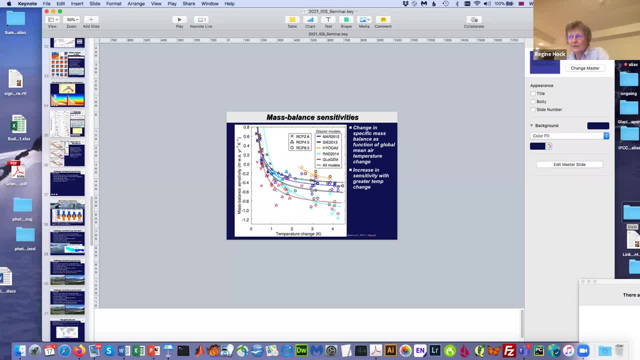 this year there's really data coming out from real, from lasers around the Arctic. Okay, great, Thank you. Great talk, Thanks, Hester. Yeah, Hi, Regina, Great, really good overview that talk. So my question for the overall 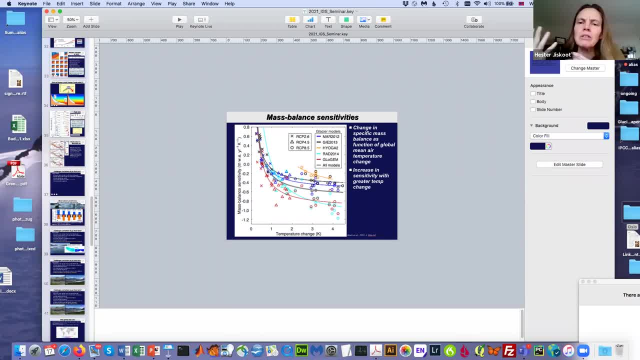 picture doesn't really matter, but do you have any idea what the uncertainties in both the glacier outlines and in the DEMs are relative to the uncertainties in the models? So obviously it depends on the, on the size of the region. So New Zealand just has a new complete glacier. 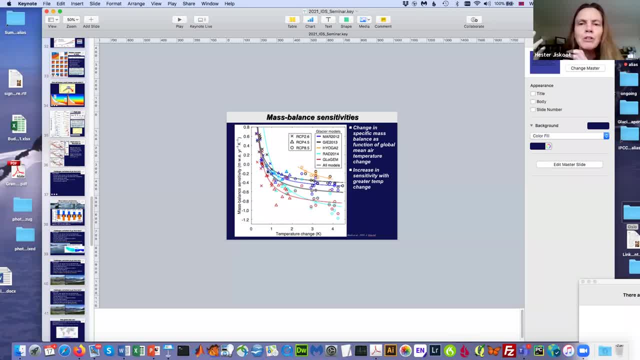 inventory And for that region it makes a big difference. but if you rerun the model it probably doesn't. But there's also some issues with the glacier inventories outside the ice sheet. So the Greenland ice sheet. it's always unsure what is part of the ice. 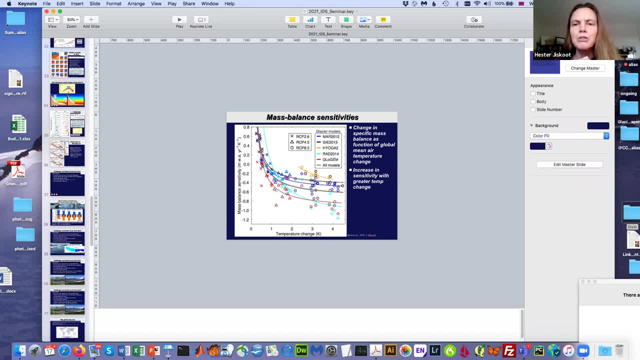 sheet and what is not. So there's some large region problems there too. So can you speak to that? speak to that? Yeah, I mean the outline, certainly like in this uncertainty analysis that I showed, that did not include any, that didn't include that part, those uncertainties, Where is it? 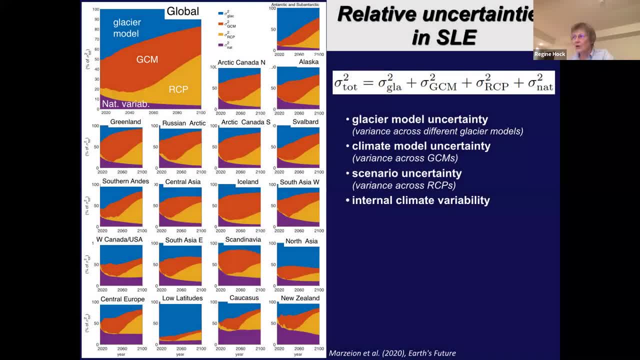 Here. So we only looked at these uncertainties because this is what we could do with the ensemble that we had, that we had so many laser models and GCMs but we didn't have like model ones with different outlines. So I would say that there is an uncertainty, but it hasn't. 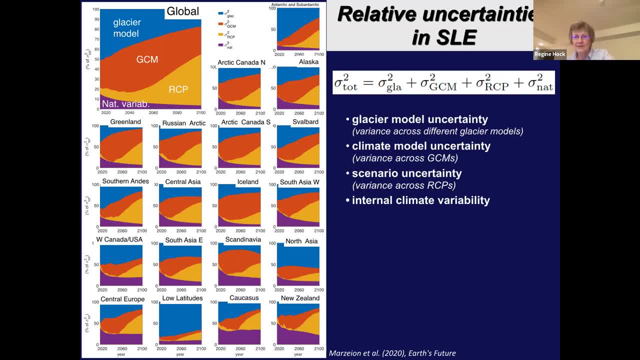 been quantified? I don't know. And then can I do one. I basically want to say to everyone that the Pfeffer et al paper, the 2014 RGI paper, has just become the best cited paper of all papers ever published in the journal Glaciology. So we've just surpassed. 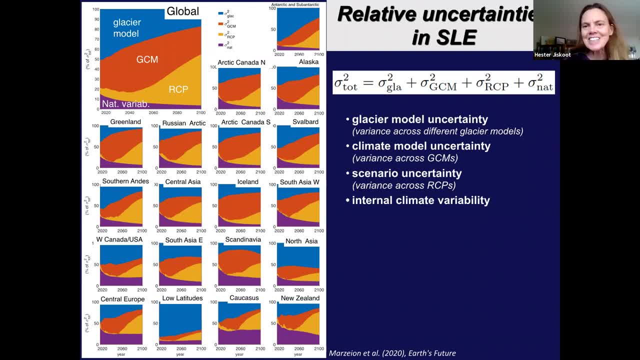 some of the classics you know- Nye and Wiertmann and Shrave and things like that. So that was an enormous effort to actually be the start of this whole global modeling. Yeah Well, that was really essential to have the RGI. Thanks, Esther. We have a question on Facebook from Todd Groves. 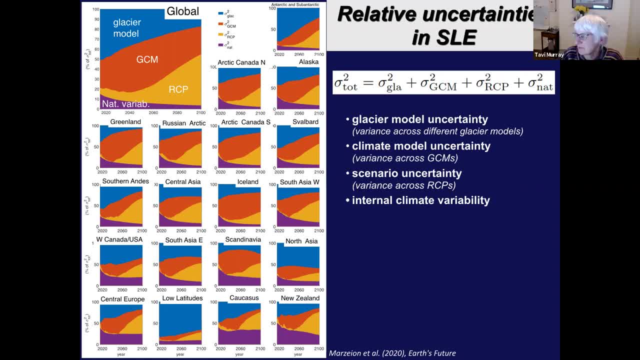 He wrote, who says I'm very interested in dead ice environments versus active ice. Do any models account for differences in the ablation zone? No, And Ian Evans has got a question. Yes, Thank you very much. That was great. I just wonder if you have any. 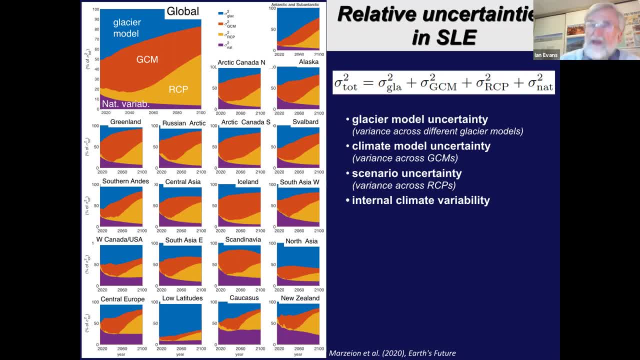 updated estimates for ELA sensitivity for the change in ELA degree, change in temperature in different climatic regions. That is a great idea. I mean we could extract that from the models. but I don't think that we have that. Maybe we haven't analyzed it. I don't know if anybody has, But in principle 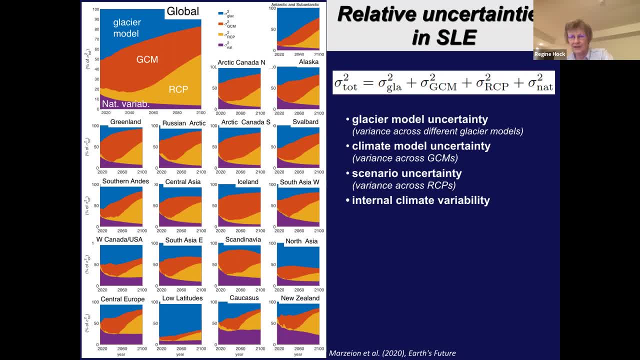 we could. That is a nice byproduct that of course comes out of the models, So one could compile that. That's great. Thank you very much. Yeah, But we haven't done that And I don't know know of any study that has done that. Nor do I. We have a question on the Zoom chat from Tetsuo. 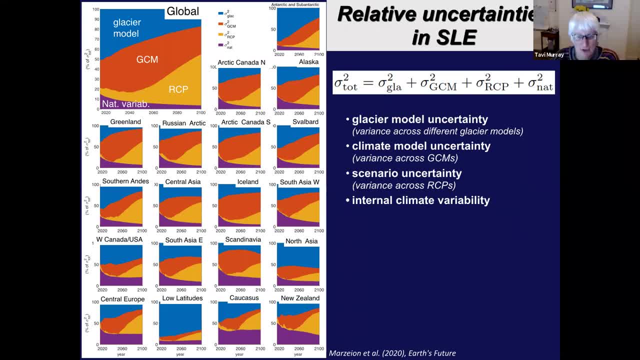 Tsuriarsky or Kaiko Konya. I'm a little unsure how the naming goes there, because there are two names mentioned in one. I might add to the last question here, actually the paper by Matthias Hus from 2015,. there is a figure in there about the changes of the ELA. There is actually one. 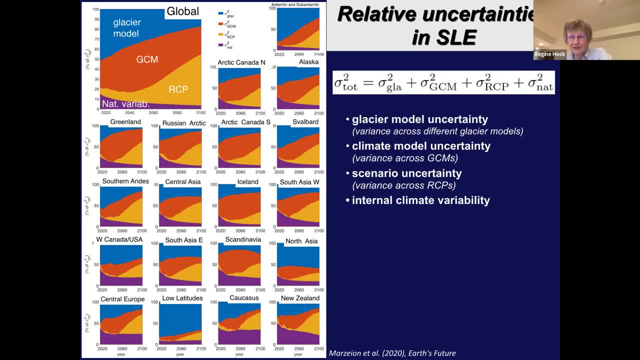 paper doing that, The ELA's in different regions. Thank you for reminding me. Great, I'll check that. Kaiko Konya, Tetsuo Tsuriarsky. So the question is retreating or thinning. So we have印 at the impression that 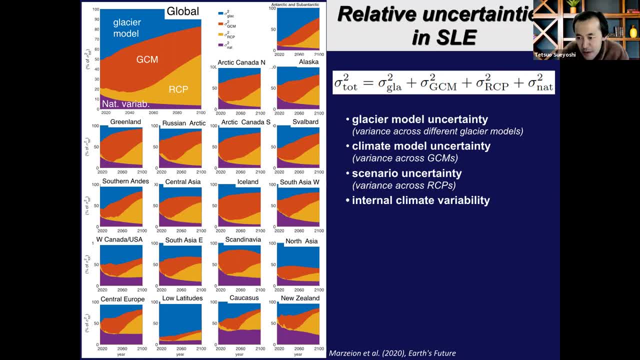 the ice cave begins, are oneガ antidote for purple salt. first, because how is it Binck得 сцен제 탊 ter하기权. Subtitle by Person名 James Brown. Subtitle by Person名 James Brown. caps should have the mixed characteristic. I mean both retreat and thinning. So I mean how many? or? 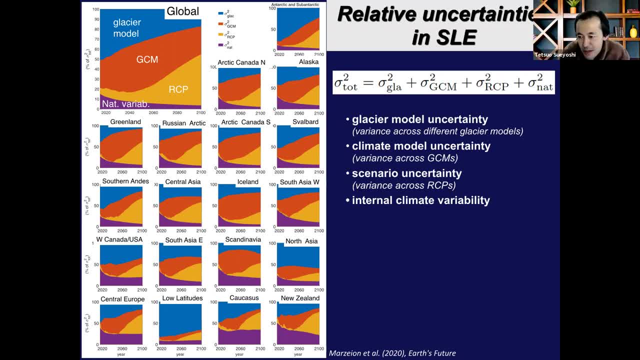 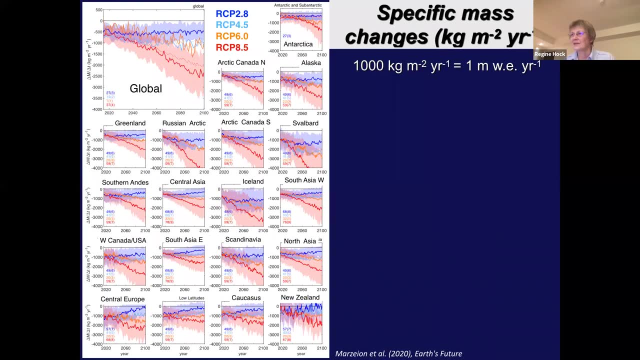 how much ratio of the ice caps show the typical thinning responses? Are they only Greenland and Antarctica, or also other ice caps? Let's go back to this. here I mean all regions. I mean it's always a combination of the retreat and thinning effect. But I think really the explanation why we